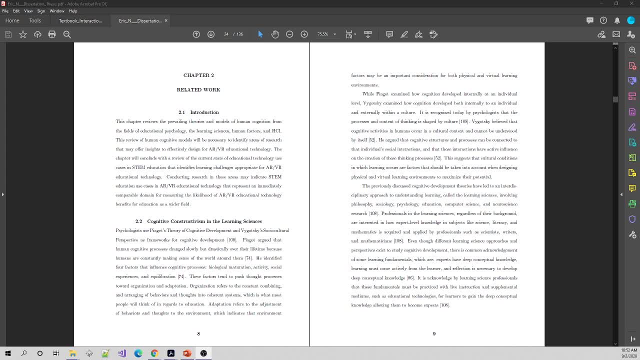 related to what you're trying to research, that you're not often left field by yourself, that there is a lot of grounding, Research has been done before you And that there are interesting areas that have yet to be examined, which means that your research. 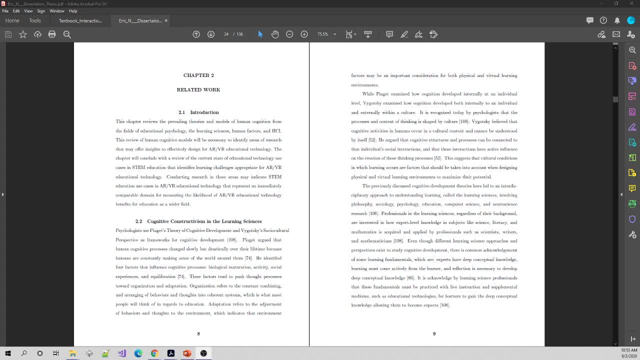 area is worthwhile. So a lot of my related work talks about these kind of grounding areas of learning, science, educational psychology, and then leads into the benefits of educational technology, specifically within STEM education. Obviously, we've got a lot of When you wish to pick a topic. education technology is helpful to all education, including other areas such as liberal science or liberal arts and humanities. 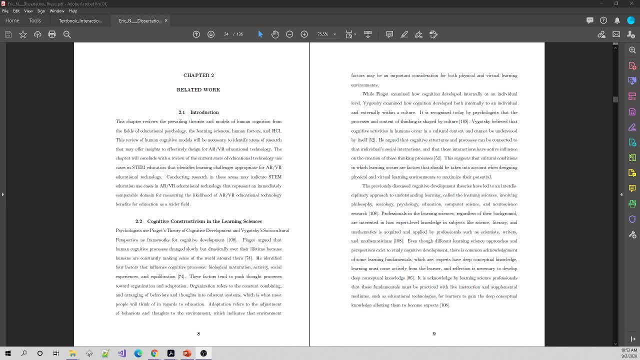 It's just that we happen to be in a STEM school with NJT, and my focus was on computer science and STEM education, So learning science is a very hybrid field. It's actually very similar to- instead of saying, user experience and human-computer interaction, which are very similar fields. they talk about the design side of software. 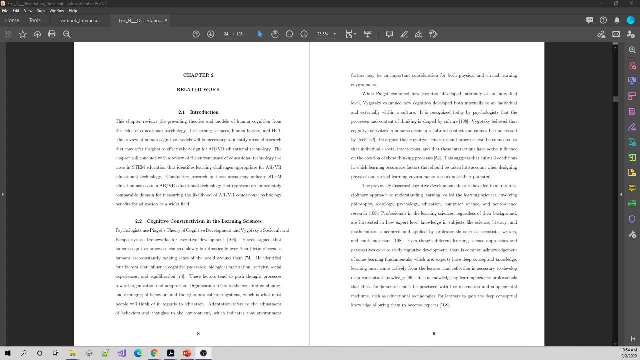 Learning science is very similar to UX and HCI, So actually this class is very beneficial to just general software design and engineering principles as well, And the better that you can ground a user, a computer user, in your software. You know, using these learning principles will help you with your other pieces of software that you build. 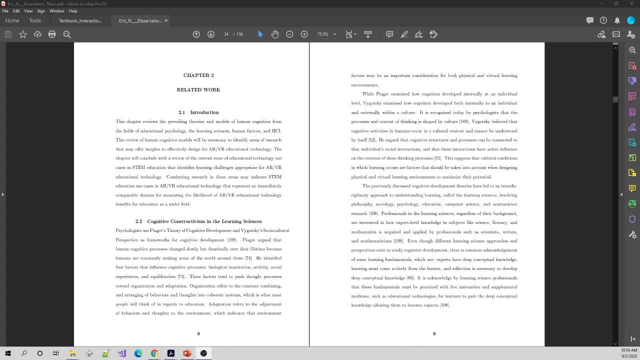 That's why games have like a tutorial level at the beginning. You have to train the user in your interactions and the computer input that you've designed for either your game, your simulation or your software. So these kind of are universal. There's a lot of overlap. 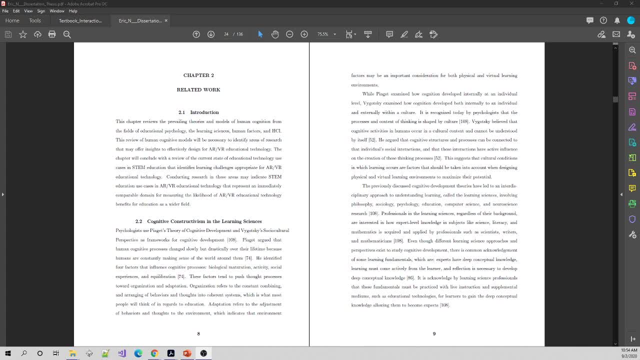 So the field of learning science is very hybrid. It hits upon psychology, It hits upon when I say pedagogy. pedagogy is the science of teaching, So it hits upon pedagogy. It hits upon educational technology and software design. 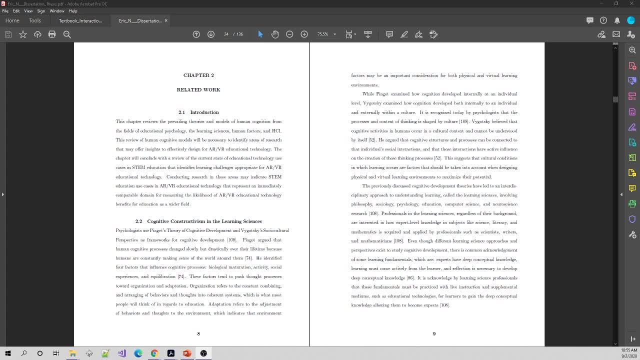 It hits upon anything that's needed to figure out the human psychology that's necessary for development and learning and teaching of people. So technology is It's super useful in this field. Obviously, the traditional methods of lecture or teaching are just a passive component, where the student sits back and just listens to somebody who's just a little bit more experienced and trying to break down the knowledge area in a simpler way so that it's easier to understand and build up the own student's understanding. 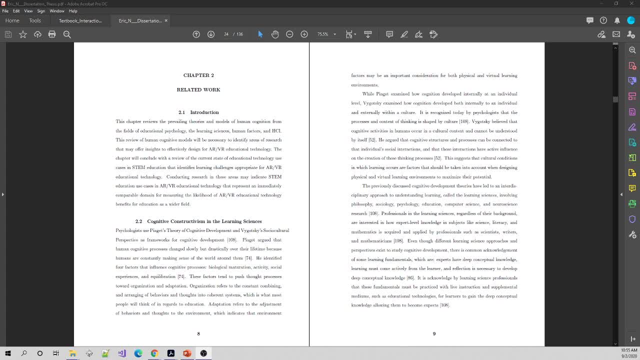 Actually that is a big educational theory in the field And it's called construction theory, It's called constructivism And it's the idea that the learner is active in building the thoughts, building the understanding in their own head. So you're going to get students or learners or users of your software that are of all ages, of all different experiences, understandings specifically to the domain that you're trying to teach, different emotional backgrounds. 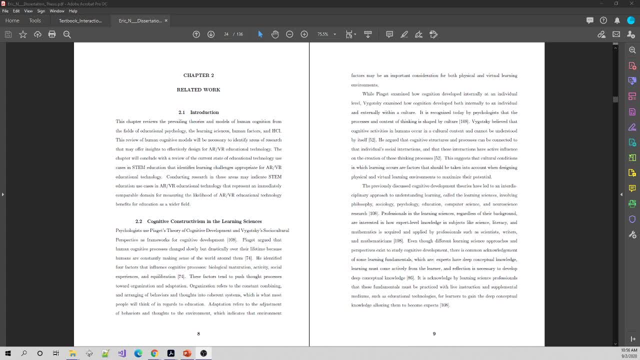 They bring a lot to the table when they're trying to learn in this kind of bi-directional relationship where you're trying to teach, so in this class i'm going to be the teacher, you're the learner, but you're trying to be learn to become a teacher. you're learning how to make your own educational technology to. 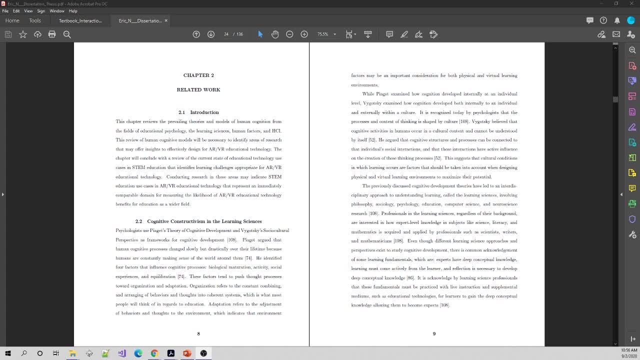 teach something, um, and so the big, the big people in the field, um, anyway, in this, this section that we'll focus on in this class, we'll use the educational theory of constructivism, which is also the primary uh theory that's also used in learning science, um, and one is the kind of the 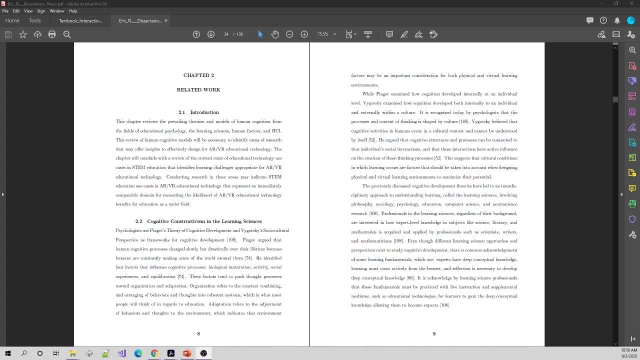 individual construct, cognitive constructivism, which is, um, focuses on the individual, what i was previously talking about, what you bring to the table, how you build your own thoughts, um, even a very passive mode of lecture, in this case through a video. technically, you could say that this video is educational technology. it's just a very simple form of it. it's a very passive. 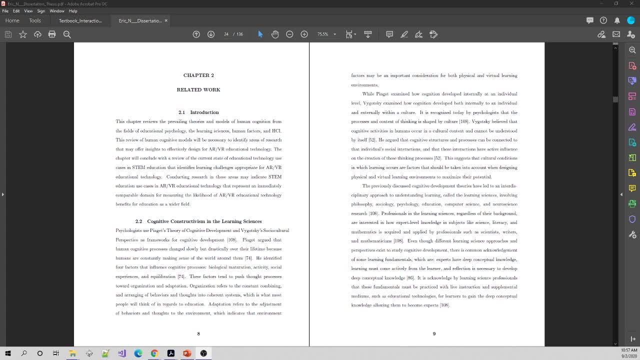 form for the learner, but you're still sitting there and actively absorbing sensory information into your head. you have the visual information coming through the monitor screening to your eyes. in this case it's a static image, not much going on, but you're probably reading the text that's on the screen as i'm talking and you're um finding interesting. 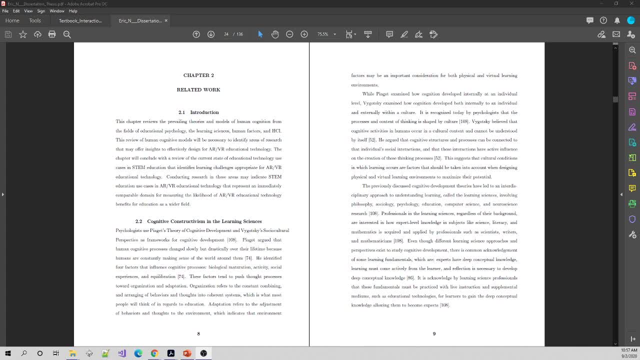 or trying to find something of interest in the writing as i'm talking, so you're receiving visual information as you're listening to me, every audio information coming through the speakers that are going through your ears, turning into electrical signals in your neurons, and this, this, i'm using a language that's developed, called english. that, and most of you, this is your primary. 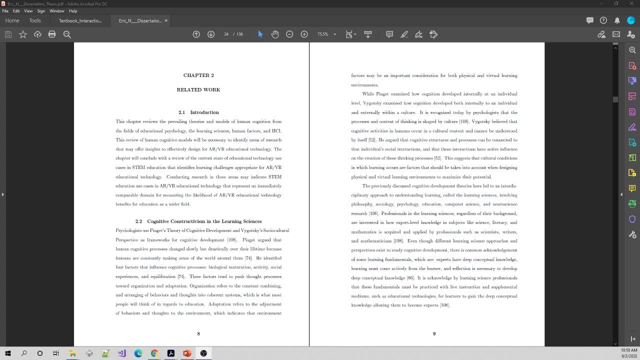 language, or maybe it's your secondary language, but you can understand, um, the ideas that i'm trying to express through my mouth, through your ears, and trying to form these ideas in your head of of of building this, this class, uh, um, this structure of knowledge that this class is meant to present. 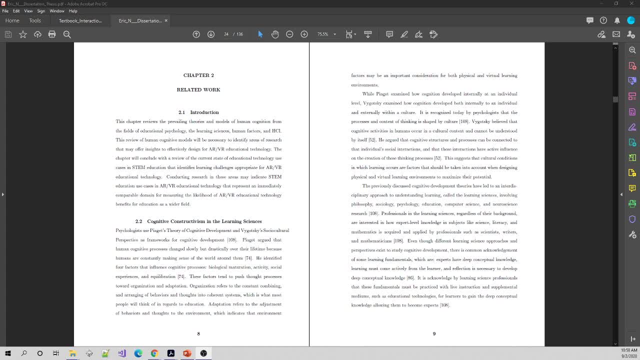 to you. and so here's: we're just in the primer area, we're just in the, the basic area. i'm trying to give you some basic building blocks of ideas to start to build more complicated ideas and actually build pieces of technology later on in the class. so you can see that i just 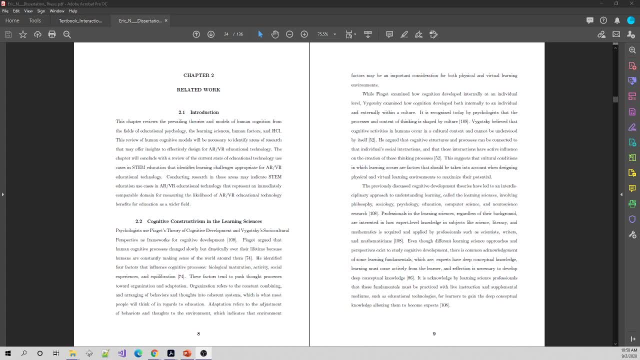 kind of expressed um, the, the psychological notions of constructivism, um, and actually i was also expressing the ideas of sensory information and input devices and um, input, um, you know the senses um on your side, through to your cognition. so i've actually started to interlace the ideas of 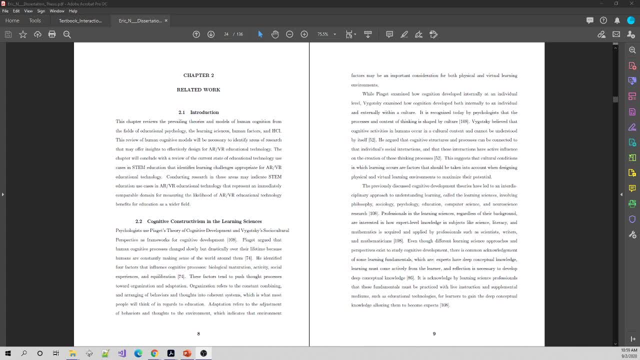 ux or hci, with learning science, and so when you think of input hardware from the computer or output, um, we're already actually kind of moving ahead into these hci frameworks where we'll talk about the software side of it. but in any case, we have the individual yourself. 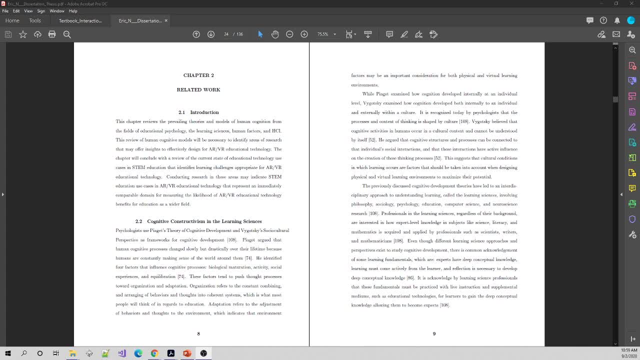 building knowledge in your head, that i'm trying to make it the most fluid, smooth process to build these ideas. so this is the idea of constructivism: you are the active builder, the active construction of building these abstract ideas in your head, and the class is supposed to be the structured time that you can. 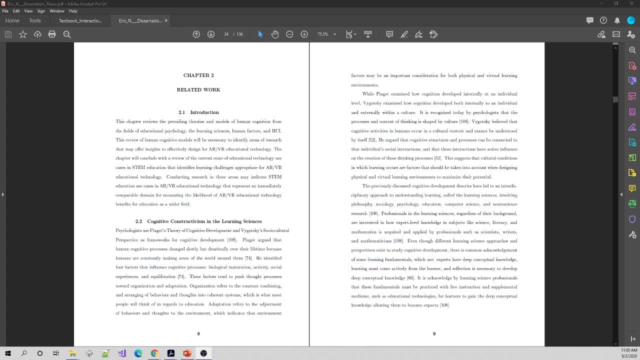 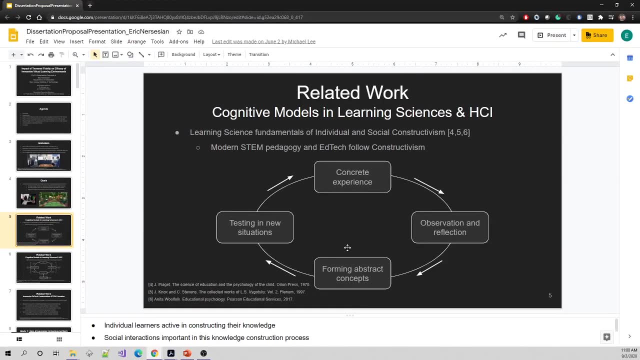 do it as best as possible. so you have this idea of learning and practicing. i do have this one graph- yeah, i'm just going to bring this up over- so i have a lot of these presentations that, um, i'm actually going to assign some of my presentations of the research we've done. not only does it, i think it does. 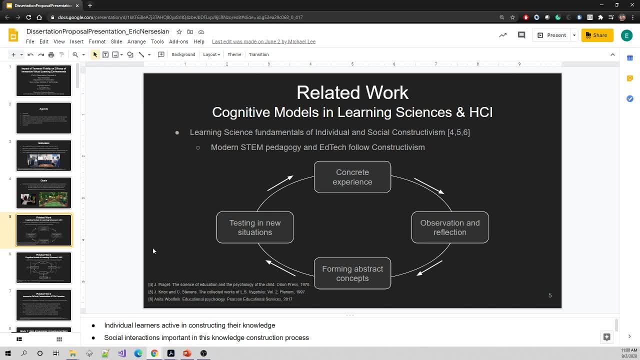 a good job of explaining educational technology, but it's like a full cycle of research on ed tech, that, um, that you can at least start to see the bigger process of research, design, development and cycling over and over and that. but in any case, this is a good graph to show. 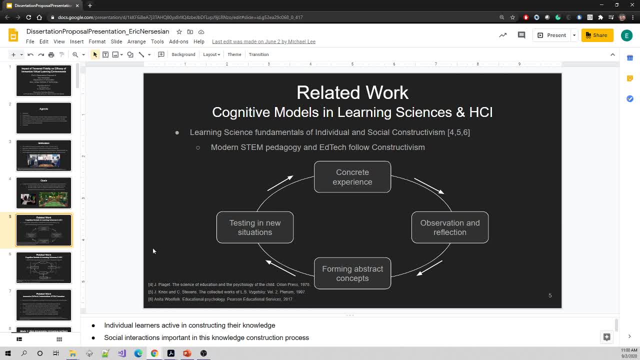 what i was talking about with constructivism, um, which is, uh, the individual or the cognitive form, as pi got and it's um, we have a concrete experience. this is from the, the user's perspective. so there's some type of experience. you have some type of sensory information. usually it's a combination of 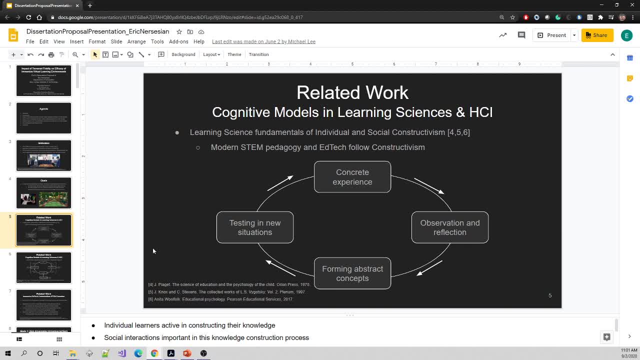 visual, auditorial, maybe haptic, maybe feelings, a sense of temperature, a sense of pressure. maybe you're actively doing something, uh, like learning how to do woodworking, your it are some type of trade, or even programming. you know, you have that tactile response. you do have to learn how to use. 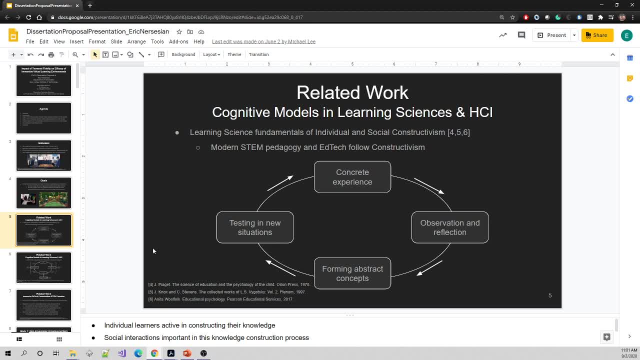 a keyboard and interface with your hands as you're thinking about your programming. so there there's also this idea of a haptic or a tactile element of the experience. and then, obviously, the abstract: what's going on in your head, your, your set, your sensory information being turned into your. 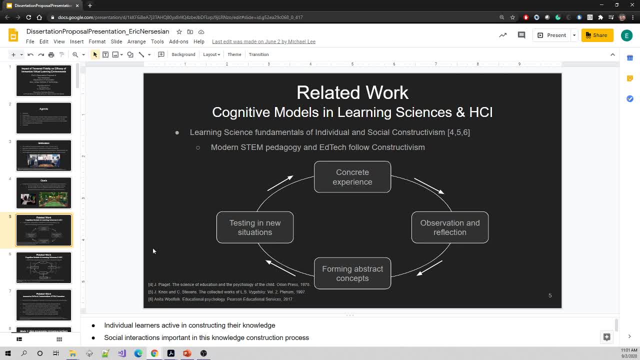 cognition, your thoughts. then you make decisions or actions or behavior based on that. so there's some experience given to the learner- in this case a passive educational technology called a video- that a lecture is happening. you are having observation, you're observing this and you're reflecting on it. what do you think about it? you are actively building these thoughts and it's a 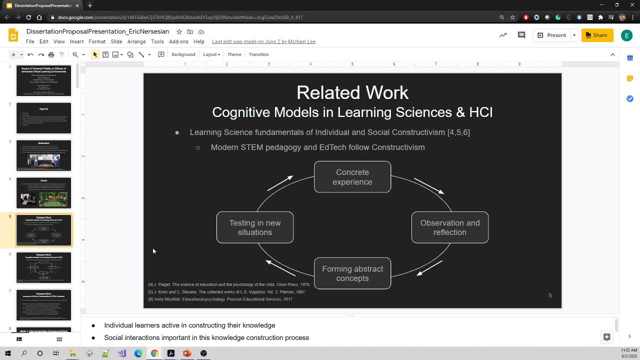 very iterative cycle in your own head of trying to match your own inner logic, your own inner ideas and cognitions to what i'm talking about, and you keep kind of adjusting and adjusting your ideas to what i'm saying. sometimes the lecture might, you might be in a, the learner might be in a disagreement too, and you're just not able to. 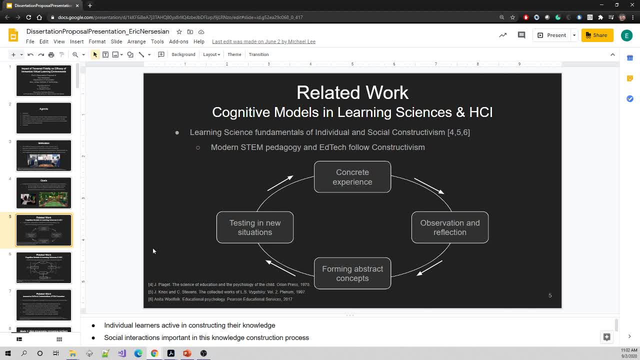 align your thoughts to it, but it more generally. these are in the normal sense of general education, whether it's art or science. you know the learner. it's a pretty, not a um, an. what do I wanna say? an argumentative or a controversial idea I'm trying to teach. these are ideas that 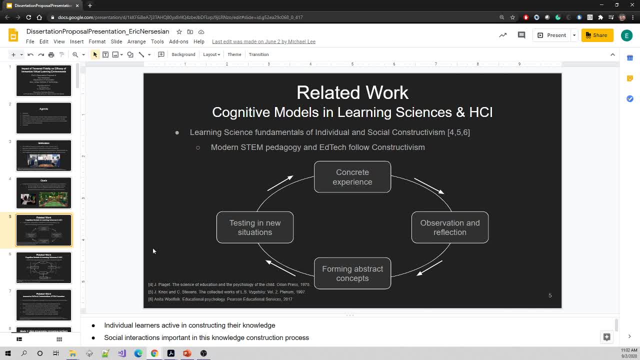 more likely you're. you're observing, you're listening to me and you're reflecting. you're adjusting your inner ideas to me and there's not like a co, there's not a cognitive dissonance. you're not in disagreement with me, so you're reflecting, adjusting, observing. 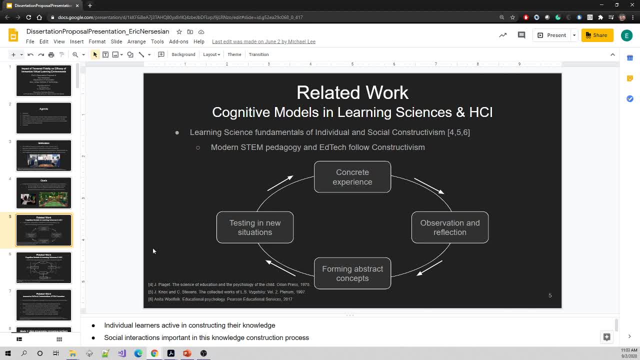 and we go on and you're forming these abstract concepts which i was talking about. forming these abstract concepts which i was talking about to once again, it's important to take that training, these ideas in your head, hopefully in agreement with me. and we knew, after learning practice, you test these in new situations, so especially in the 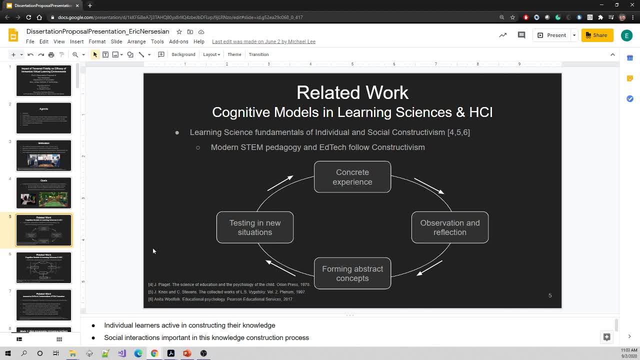 technology schools. we are all project oriented classes and I'm going to be building a project for this semester. I'm going to be showcasing previous projects that we worked on this, mostly the C Spresso, this using virtual reality to teach computer science and math concepts to younger students. but I will 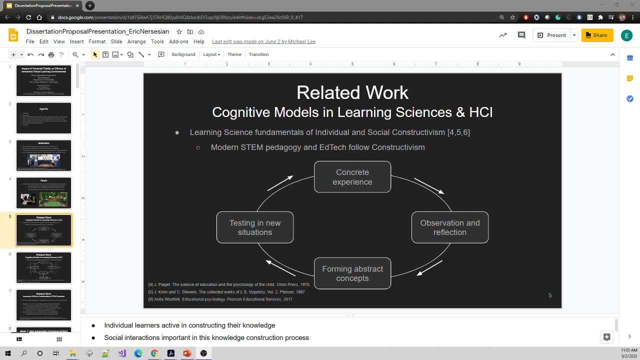 be building, going through all the phases that you will be in this new project that Jess is working on with Hannah over in in co-ed that you might know called the Canaan project, and so we'll do a very small cycle of research, design and prototype along with you of the same scale and scope, so hopefully it's easy. 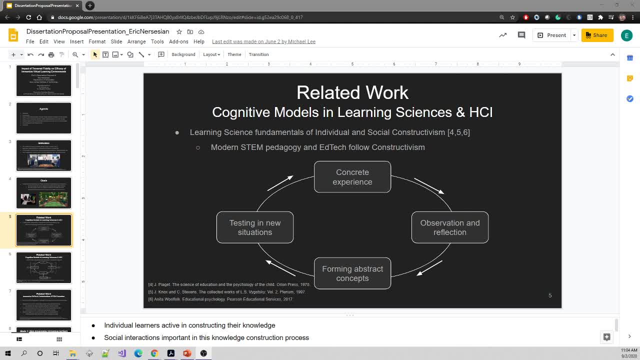 to follow along yet with your own ideas. so, anyway, you're going to be testing in a new situation. practice is always, you know, fraught with I'm gonna write off the bat. say: failure be, and it's not a bad word, it's a very good word. it means you're gonna learn. so you know you fail. 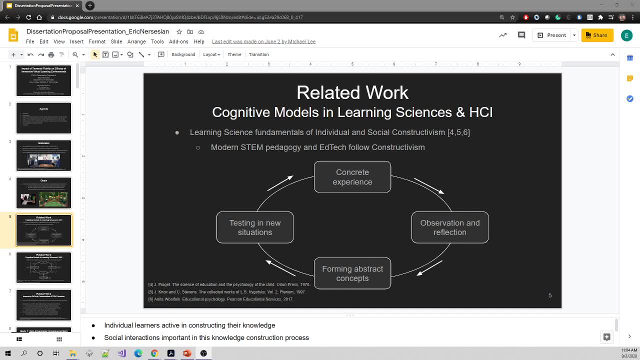 a thousand times before you succeed. you know, Edison said with the light bulb. and so that's good. we want that, we want practice. you're gonna go through all these rabbit holes and tangents of thinking and testing and prototyping and you're gonna come out with something. 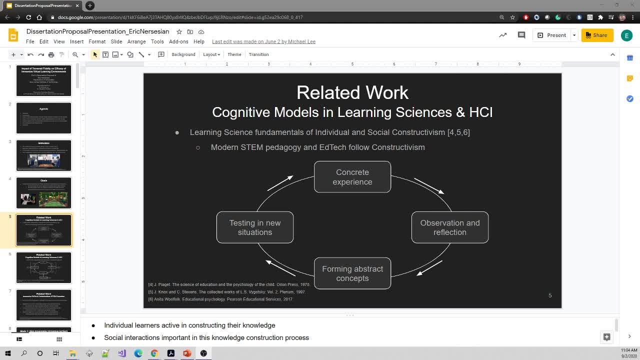 at the end of the class and you'll be able to build a portfolio piece around it. and it's okay if you made some wrong decisions or inaccurate, or what you thought in hindsight at the end of the class might have been like: well, I feel like I could have made a better choice at that point. that kind of led me down a. 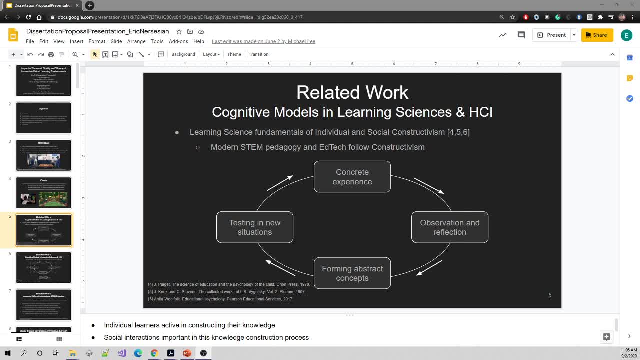 different path when I finished up my prototype. it's okay, it's still a worth, very worthwhile process and you will still have a great portfolio piece and you can return back to it and just go through the cycle again at a later point, even with even stronger skills, and make stronger portfolio pieces. so anyway, you will be. 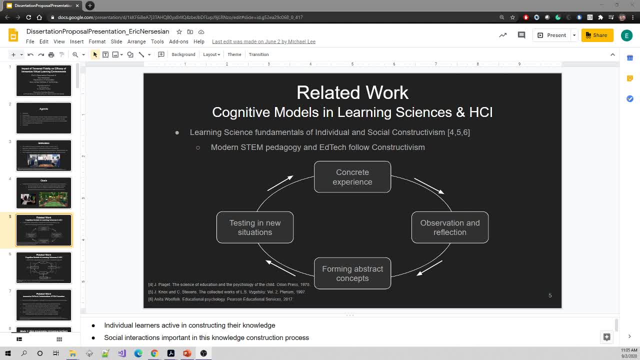 testing and we return back to another experience. so we either have to return to the same learning point if you need another cycle of learning and practice before you get it, or we learn on, move on to another point, maybe a more advanced point that we first needed to cover the beginner point, or we go on to another. 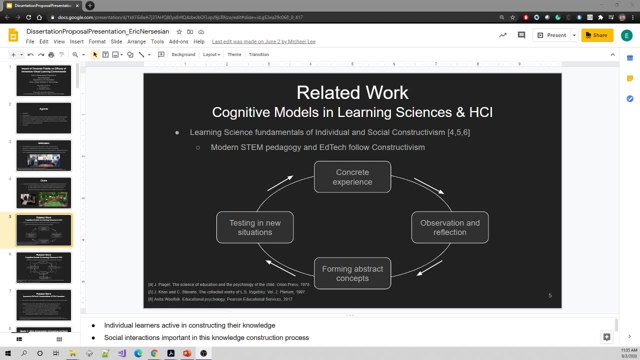 topic, or maybe you have a question and we explore an area that you're interested in, but, as you can see, life itself is very iterative. the learning process is very iterative, and that's why software development itself is also very iterative nature to it. so, all of it, we're always cycling on. in fact, I'm 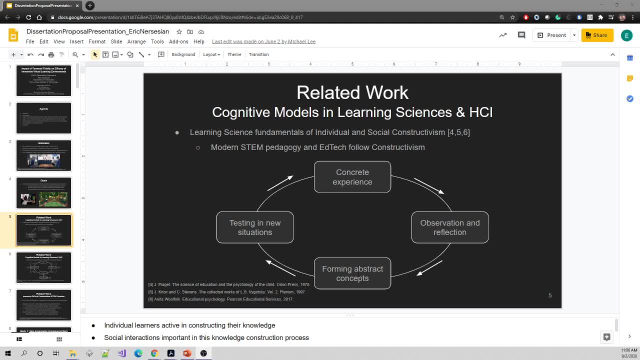 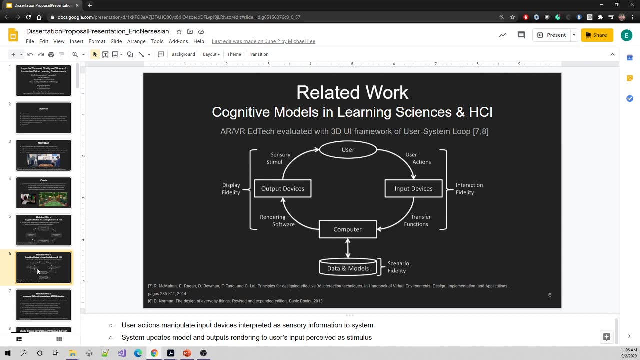 going to. so this was out with Pigo, with individual constructivism. I'm gonna talk about Vygotsky in a second, but those are like the two main guys there's, there's hundreds. you know so many people have added to this field. but as long as 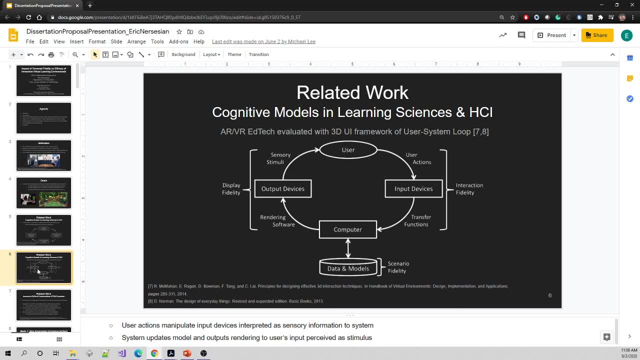 we ground you in Pigo and Vygotsky. you're good. we have individual constructivism and we're going to talk about an element of social constructivism, but in this case I was kind of talking about these cyclings and I want to just touch briefly on some of the things that we're going to be talking about in this. 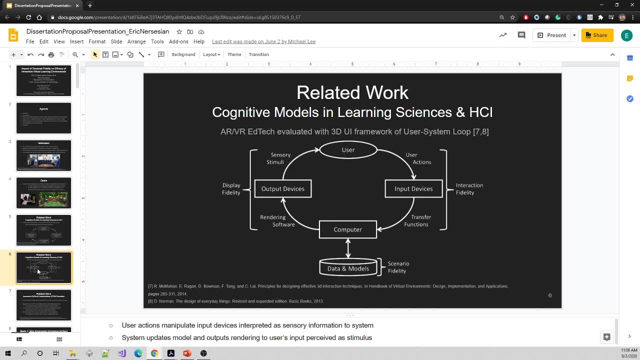 video and then we're going to talk about the. we could talk about the educational technology cycle, how it reflects over into this side, it reflects over into the hardware and software side, so that you might be able to look out a bit further and where this class might go. 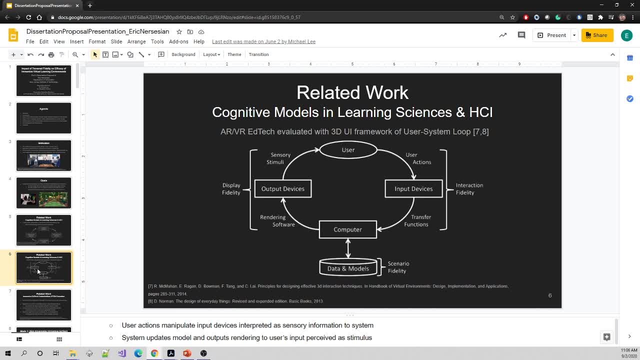 but we will be using what will be called the user system loop framework. it's very useful to. I found it very useful in my research. it is a user interface framework and I've used it for augmented virtual reality, but I like how it breaks down the interface. 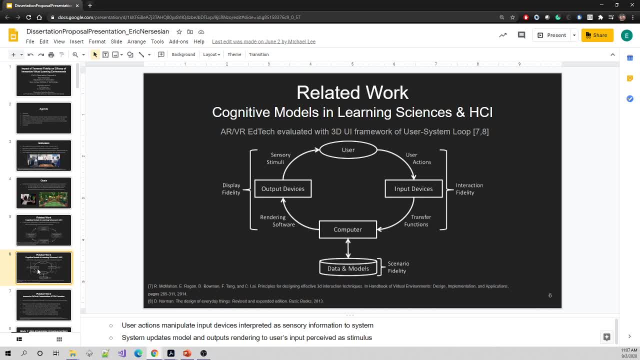 between the user psychology and computer processing site. so it's also very viable for 2D as well. and in a moment I'll talk about the bottom area. it relates well to the simulations you have to build for educational technology. but anyway, at the top we have the user, the user. 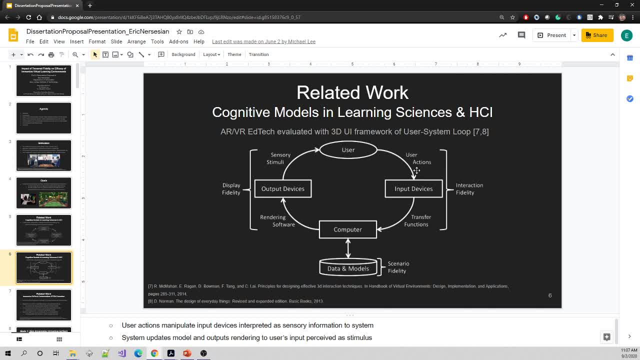 will be expressing some actions. they'll either use their hands on the keyboard, they'll use their hands on the mouse, they'll use their hands on a touch screen or, nowadays, you know, hand tracking is just, you know, just doing hand movements in the air. they might talk, there might be voice recognition. 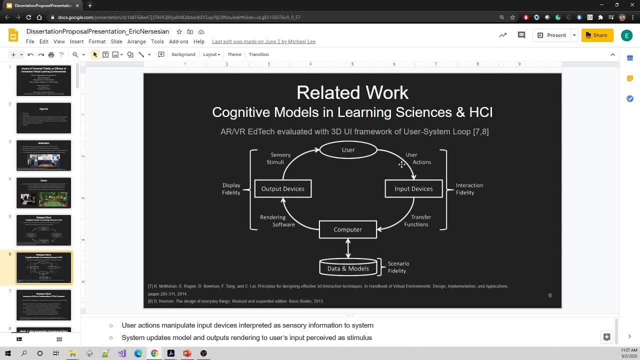 software or whatever. the user uses their body in some way to produce an action on to an input device on the computer side, and it might be a keyboard, a mouse, a touch screen, sensors looking at the hands, a microphone picking up their voice, or whatever the input device processes all this, usually analog data. 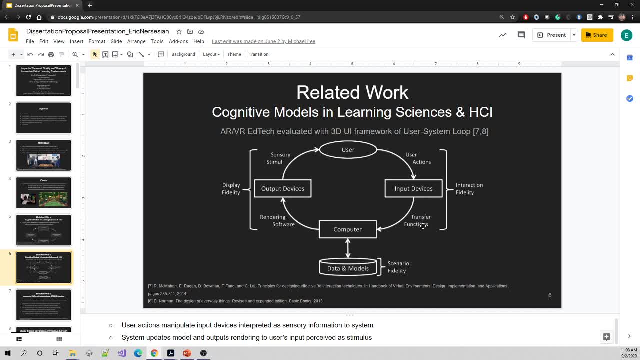 real-world and to some digital format. it does some transfer function, creates some data that's useful for the computer to process on you, you, you, and this side is called the interaction fidelity. this is the interaction design area and this is where we'd be focusing a large part of the class. how do you? 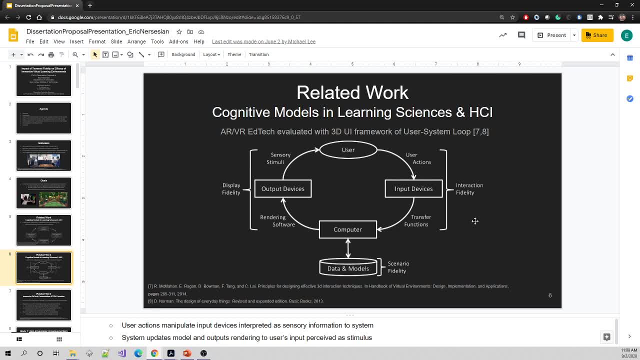 design your interactions so that they're useful, easy to understand, yet expressive for the user as they go through the learning process and then their commands are done upon the computer program. the computer updates the back-end. you could think of this almost as a model of you controller design, MVC design, and if that's new to you too, we'll have a. 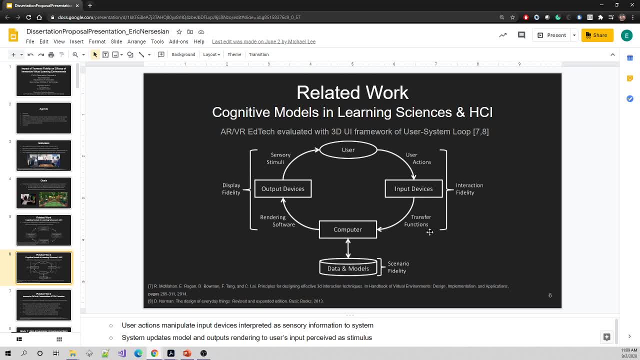 separate video on that. but this can be thought of as the controller side. the users giving has a controller element is giving command, so it's giving control to manipulate the computer side, the back-end side, or the model side, where we're gonna model a piece of reality, meaning we're gonna simulate something. 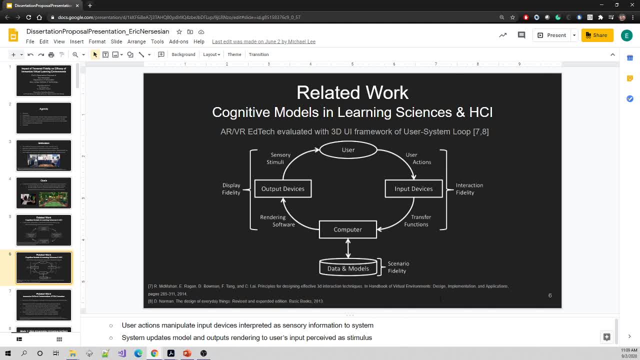 so, and this, this project we're looking at, we're going to simulate a piece of ecological geography. we're gonna wear these populations of Canaan's or live so we're going to model a piece of reality or simulated. that simulation can be adjusted, manipulated, affected by user actions on this side and the interaction. 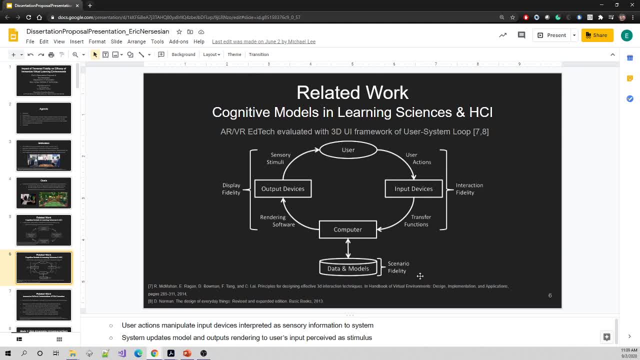 side, and this is our scenario- fidelity. how fidelity, meaning like, how much of reality do we have to recreate in our simulation? that's a fertile ground for the user to learn something. once the simulation is updated, we will update our rendering software. what will update? our visuals? or, if there's any audio, maybe. 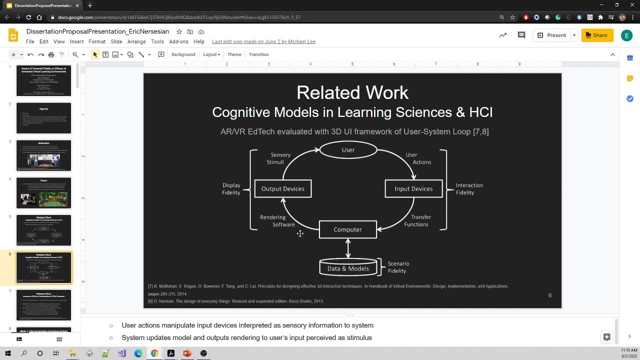 there's haptic feedback with hand controllers, but usually it's in this class it's it's going to be primarily visual. it's going to be computer graphics rendered onto a monitor, which is our output device, and that creates sensory information or stimulus back to the user. again we have our full 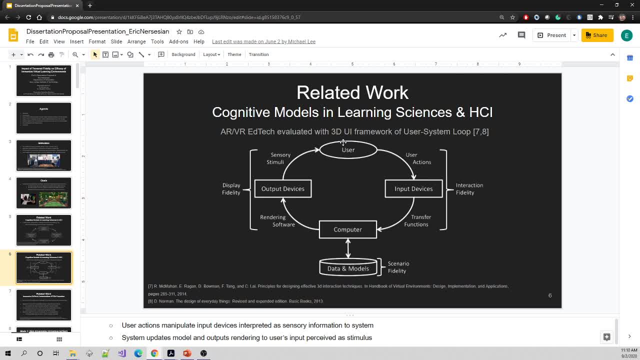 feedback loop. the user has new information coming through their eyes, to their ears, maybe through their hands, that allows them to change their thoughts, have cognition, allows them to make decisions and implement an action that changes the simulation, that changes the sensory data, the stimulus back to the user and this 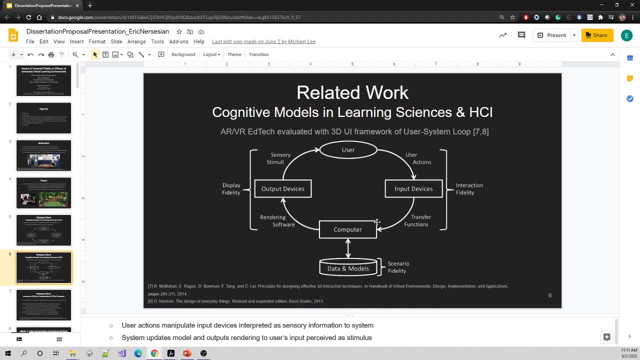 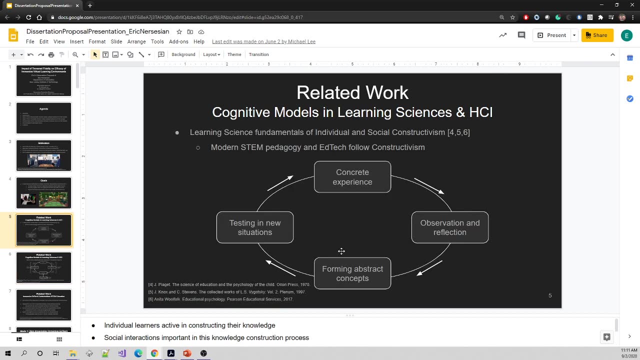 continues hopefully until we have a successful, happy learning process happening in. the user or the learners is happy in learning. it's a fun, engaged experience. so you can see at the learning process this, this feedback loop in the learning process, this feedback loop on the technology side is very 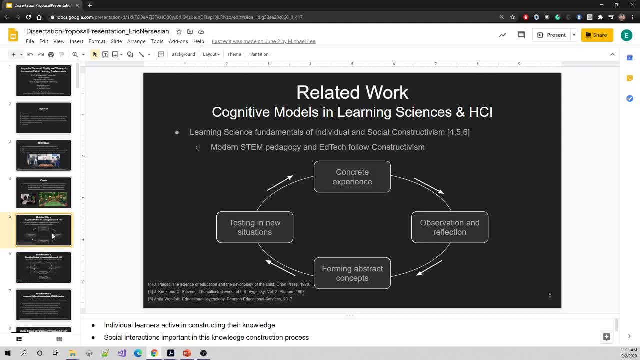 similar and that's why we reflect upon these two processes in educational technology and hopefully you can see why educational technology might be so important. so impactful is that it almost encapsulates this learning process without the need of another person, so you can automate it. it's very tiring. 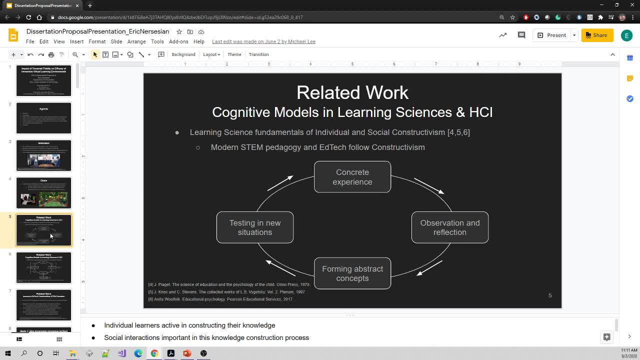 and to learn how to be a good instructor. hopefully, i'm having a good job in this class, um, and it's it's. it's tiring and but it's very rewarding to learn how to be a teacher, but you have to do it over and over again per class, which is actually why i'm making this video. 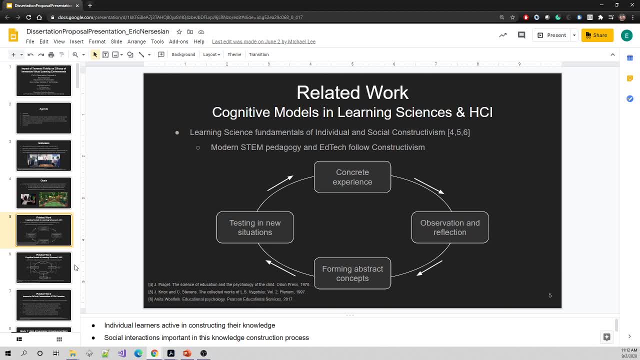 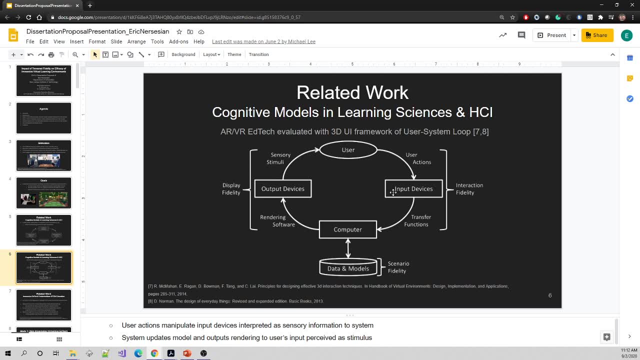 i'm actually automating my, my learning, my teaching processes and to the learners learning processes by creating this video that can be watched over and over again. you can pause it, you can return back to it, you can go take a break, you can reflect, you can watch it at later dates and i can reuse it in other classes, and so i'm taking advantage of 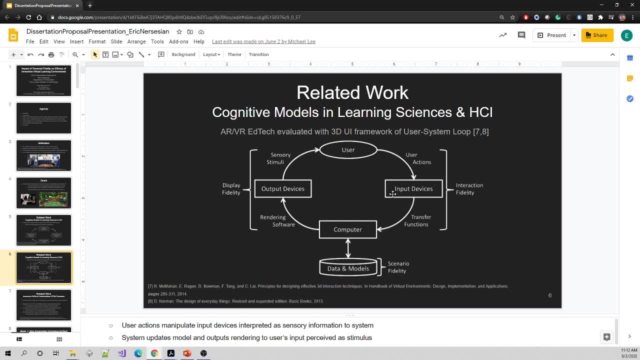 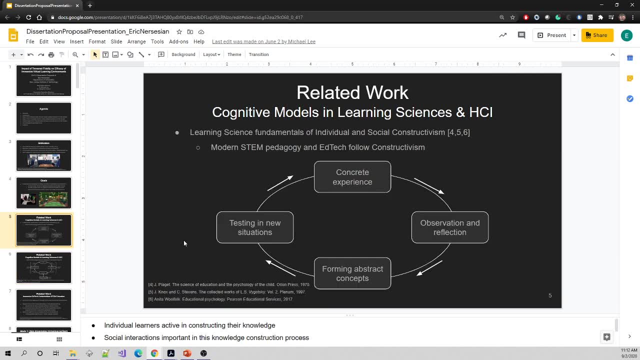 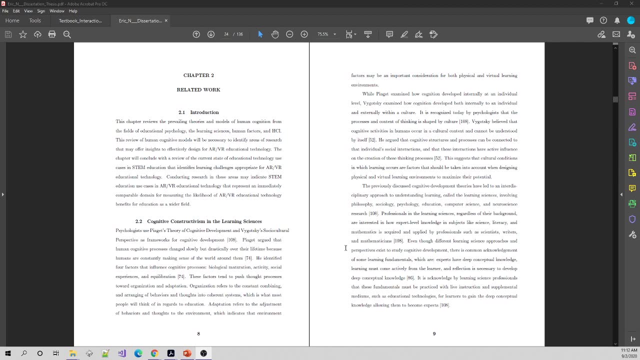 user of educational technology for these benefits, and this is what you'll be learning to do as well. so i did want to return back to vigotsky, um and finish this lecture on um the basics of learning science. so i'm going to grab out all of pedagogy and educational psychology and psychology and all of this. i'm just going to 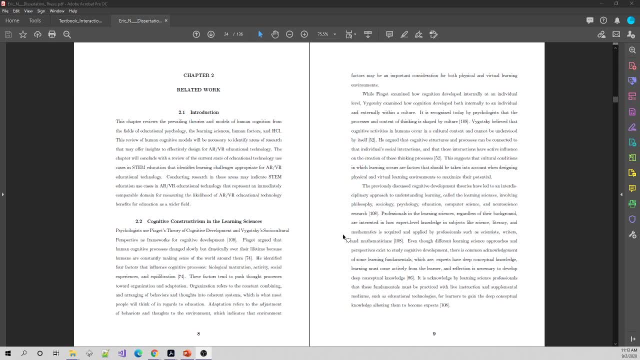 wrap it up into learning science and within learning science. i mean, that's why learning science exists, because there's so much to education, so many facets to it, especially when you bring in the idea of technology, and so they have this very big hybrid field called learning science and within learning science. we're just going to focus on the idea of constructivism. 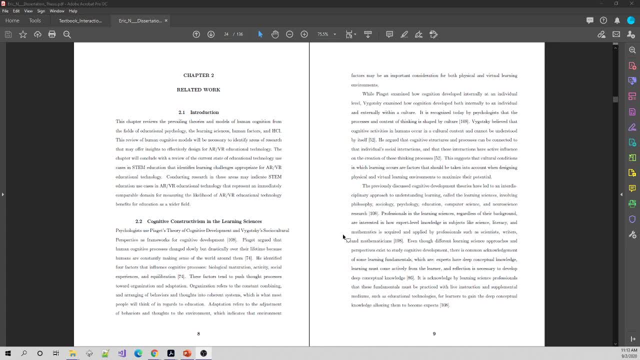 as the psychological theory of learning science, and we're going to focus on the idea of constructivism as the psychological theory of learning science and we're going to focus on the idea of constructivism of how learning works. um- and we just covered the individual side, um- with. 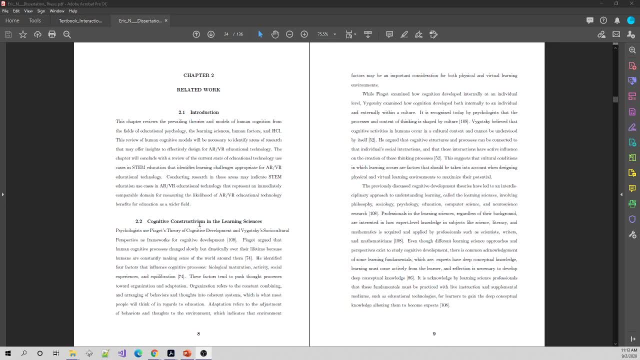 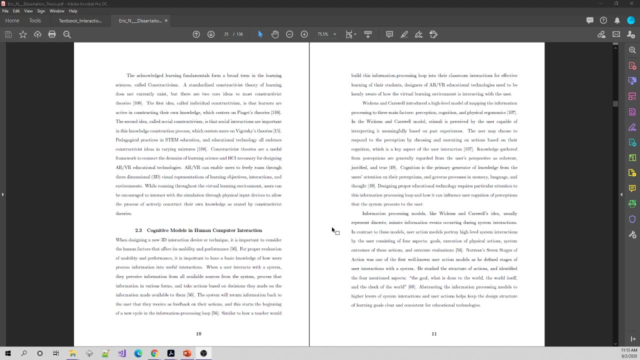 pie get if i go. i go. i write the moment. i'm sorry, i'm just tired of this baby. i can't remember. this is the pronunciation of his name: um, and then vigotsky. we have the social cultural perspective as well, so it's interesting to note that. um, i think i'm also going to 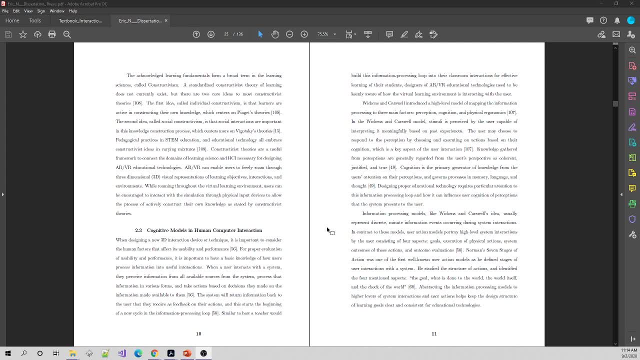 um, just um, cut out the related works section of my thesis, the thesis, that dissertation, has been published yet, so i can't give you the pdf. but i'm going to cut out the related works section and post that up for you to peruse on your own time. and actually that is a another piece of educational technology. 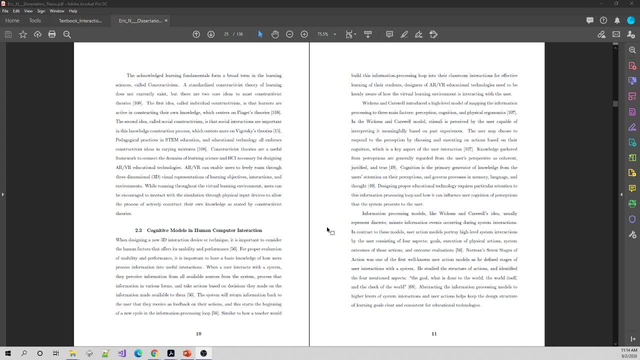 um, just kind of as passive it's. it's at your own leisure. you can read through a document, right, and it's um. it's a file presented on a computer that can have text and images and maybe even moving parts like a video or an animated gif with it. 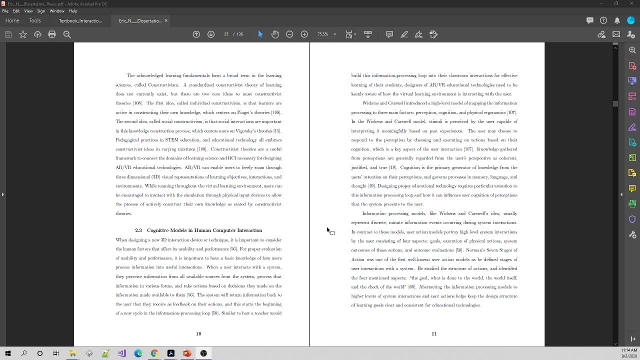 but we'll be doing more interactive simulations. you can gamify as much as you want and we are going to be talking a lot about game design, but i'm going to steer away from the the term educational games, and it's more about educational software or educational technology, because it's 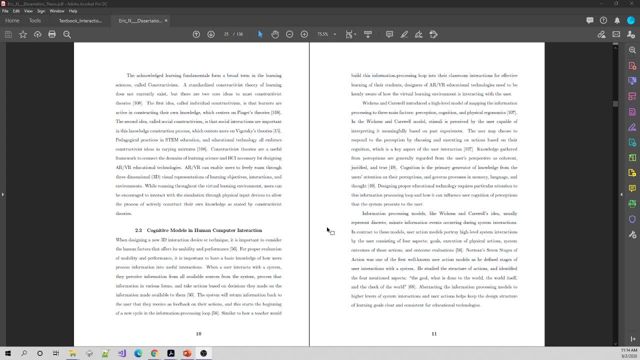 we're going to pull in everything, um, and at the end of the day it's supposed to be engaging and really fun, and we're going to use a lot of ideas for games. but it is a learning situation and it's serious, um, and so we're going to call it educational software, but in any case, um, uh, vygotsky looked at. 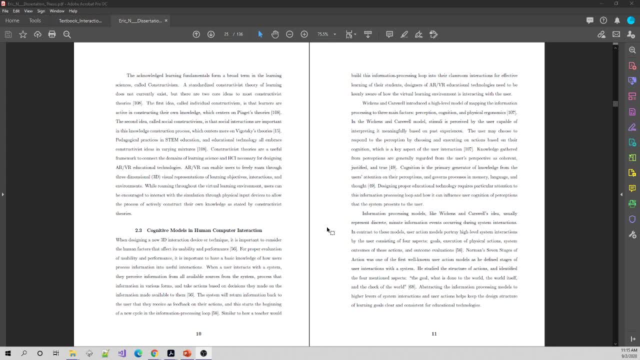 took a different perspective than uh pieget and he, and it's not um one or the other, it's the fact that, yes, the learner is self-determined, is individualistic and building. you're responsible for, for building your own neural pathways in your head and maintaining them over your lifetime to be an educated person. 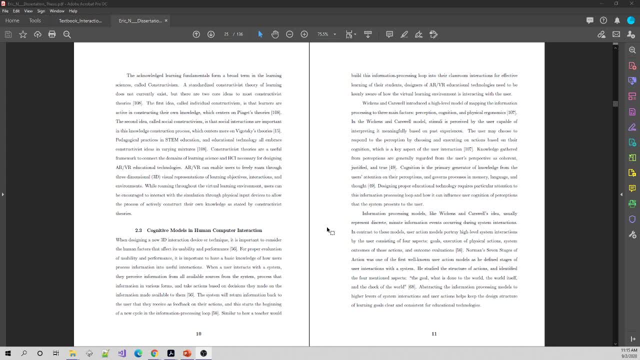 but you're also immersed and surrounded and cannot avoid culture and society. All of our learnings are through a cultural format. You learn to talk, You learn to speak, You learn to listen, You learn to see act- all these rules of society. 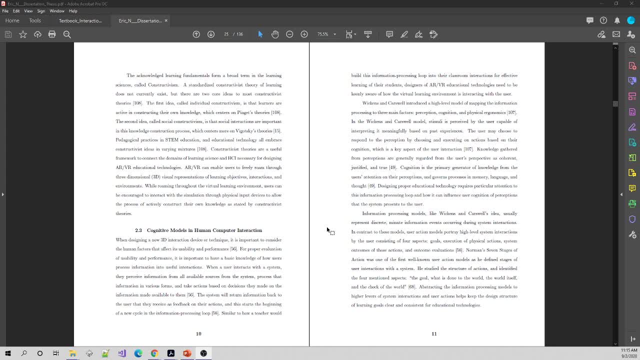 Everything we learned, all these knowledge domains that we're teaching, of education, math and science, and language and history, all of this is cultural, And so you cannot separate the learner from their society, from their social surroundings, And so Vygotsky really focused on that. 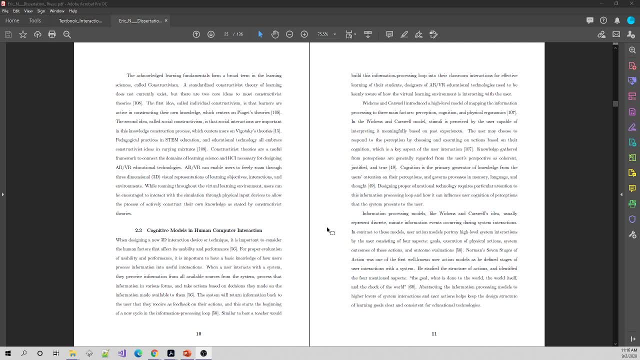 In fact, here you could say that I am transmitting information to you and you're sitting in this remote location all by yourself and listening to these electric instruments on your desktop. you know these speakers vibrating, causing the molecules in the air to vibrate against your eardrum. 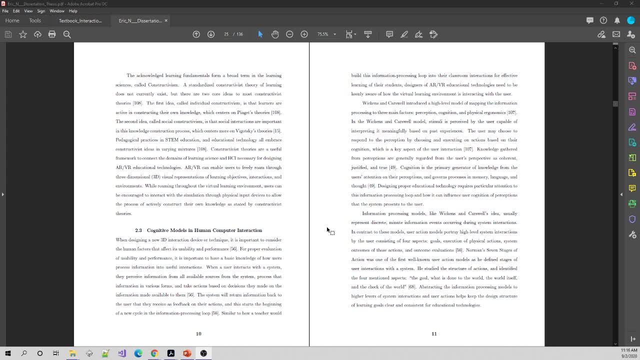 and these electrical signals that are produced. Your brain has been trained culturally to understand certain ideas that you're hearing as words combined together in sentences and larger ideas, And the fact that this, this video, is also turning on all these millions of pixels on your screen. 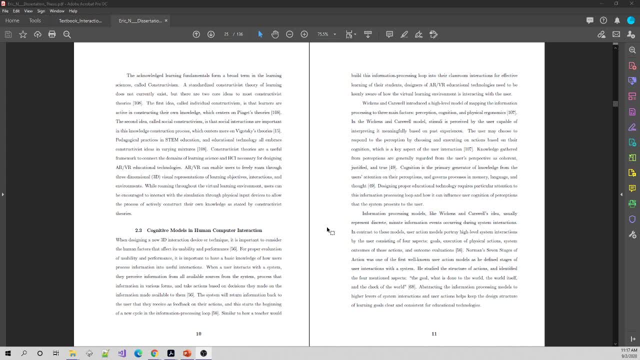 at different brightness and hues colors to create this cohesive image. It's actually not a cohesive image. It's all these pixels sending out, all these different light waves of different wavelengths that your eyes are processing, that together inside your head, somehow gets formed together into this picture. 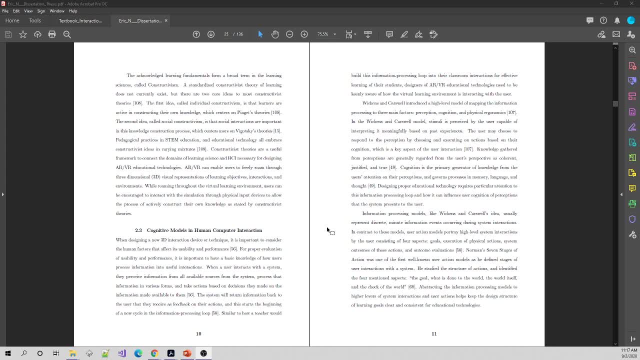 Um, that's presented to you out in reality, That's on a plane, on your computer, that your brain is processing into an image, that of, in this case, very simple white and black and these weird little wiggle lines and edgings of black and white. um, your brain can discern from previous learnings: 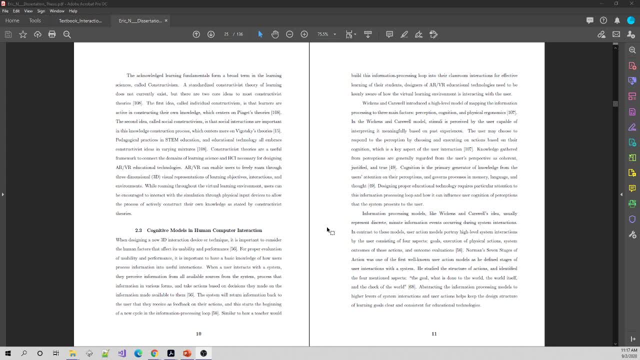 You know the previous changes in your neural network can process these black squiggles into words that you read together, That you process into sentences. So, in the same way that I'm talking and you're you're, you're processing the audio signals. 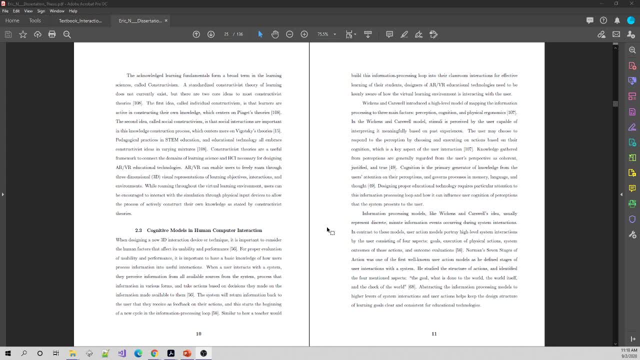 into words, that piecing them together into sentences, the same that these black squiggles you're piecing together into letters, into words, into sentences, into larger ideas And all of that. I mean, I just went off on this, this crazy tangent about technology interfacing with. 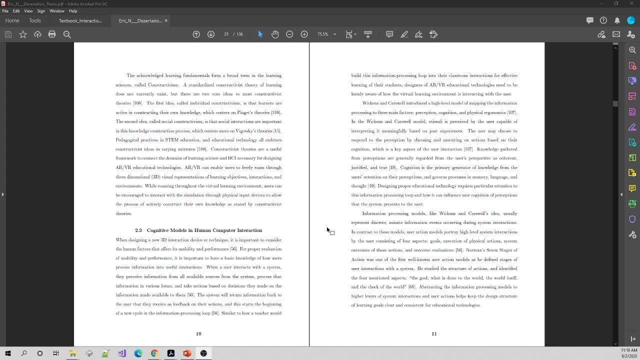 real world physics interfacing with your, You know, body Oregon sensory organs into your brain, um the cognitive Oregon, and all that having to deal with a cultural slant on it. All of that is this: you know, electromagnetic, uh, physical phenomena. in reality, that was. 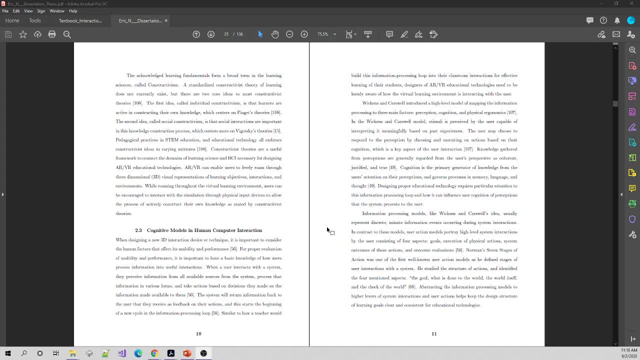 trained by human society to mean certain words, certain ideas, even the idea of language. It's just these ideas in your head. but all of that is cultural, All of that is social, All of that's been trained onto you since birth. 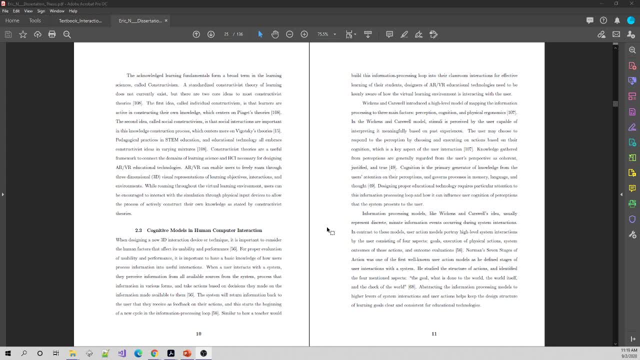 So you come into my classroom with 18,, 19,, 20 years of being trained culturally And um I you know, I do. I aggregate, I make a stereotype of where I think the average student is and what the point of this class is. 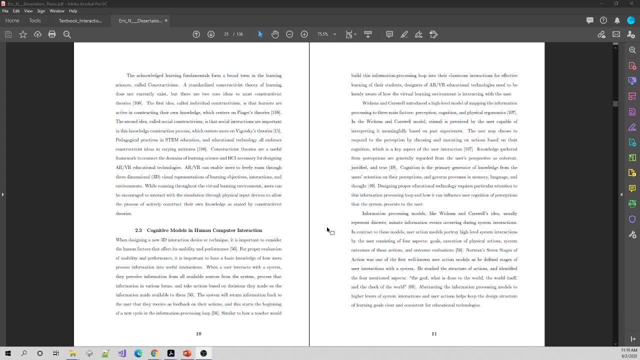 And I try to cater to the average, the biggest part of the class- but obviously we're going to have a lot of outliers and that's where we have lab time And, uh, you know, correct. So I think that there's a lot of um, like I said, um off the top of my head, like 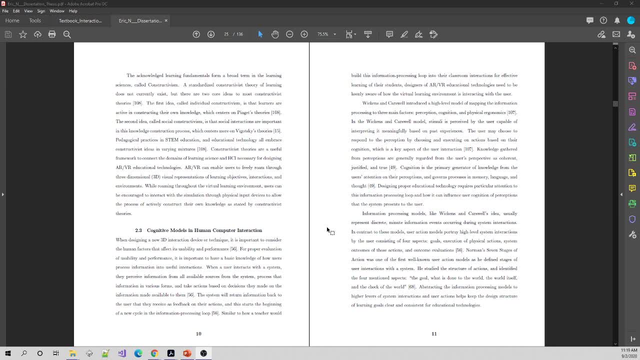 like: what's the problem with, um, everything I'm like I don't know I'm supposed to do it in my head, So I think that's something that I'm not good at. I was able to sort of put all of my knowledge and stuff into this. 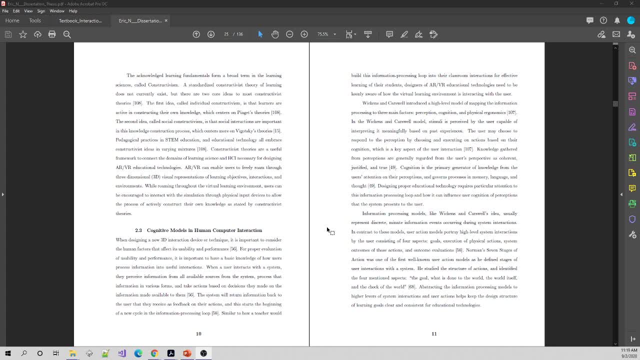 You know, I think I shared an idea with my friends when I was a student of. of course, we all need to kind of earn a living, you know, we all need to do something to live and to earn a living. But I think that I think that there's two main things that we need to do to be able. 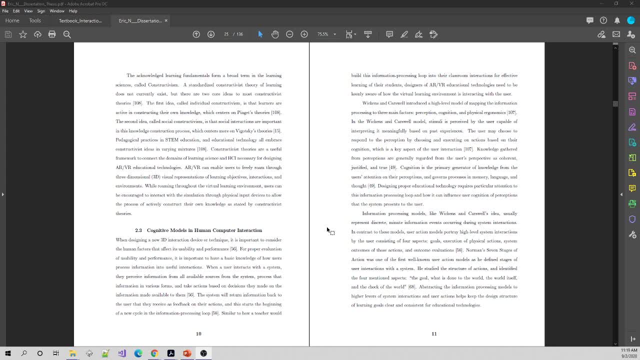 to keep our energy going and to be able to do the things that we need to do. And- and that is Yeah, Yeah, Yeah Yeah- perspective, a cognitive constructivist constructivism, or from a cultural perspective, from a social constructivism, and that's Vygotsky. So there are different frameworks. 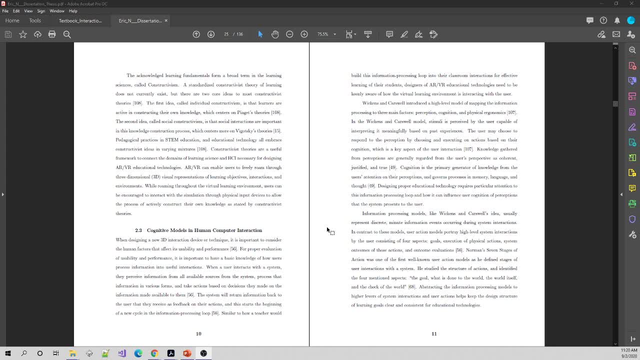 there are different lenses, to think about a learner and to think about how to approach them, to think about how to develop some educational material to present to them and to try to minimize, you know, like lost cases or worst case scenarios where you're just way off. 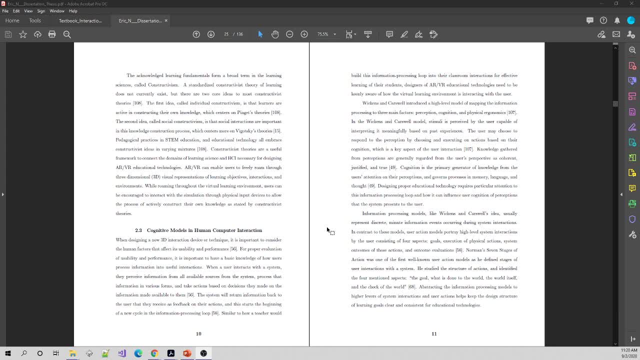 the mark. You didn't hit them directly with your approach, with your technology to educate them in some way. So hopefully that all made sense and that there's these two ways of viewing people: from an individual, from almost like a neural net perspective. 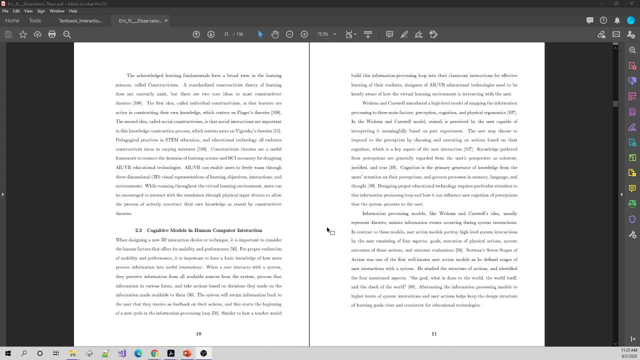 and from also this cultural like that everything's been trained through the mind and that you have to deal with somebody as a within their cultural context, and people learn best with this cultural context being socially around, that you need to be immersed in talking. 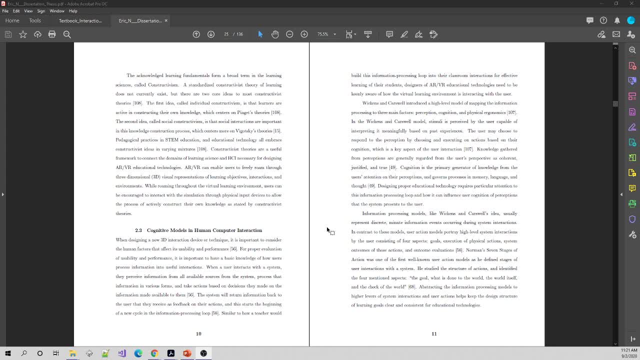 that you're listening to me, but you're turning to somebody next to you and you're talking to them and you're trying to use your own social interactions to help solidify the learning topic in your head. So it's almost like a practice part. 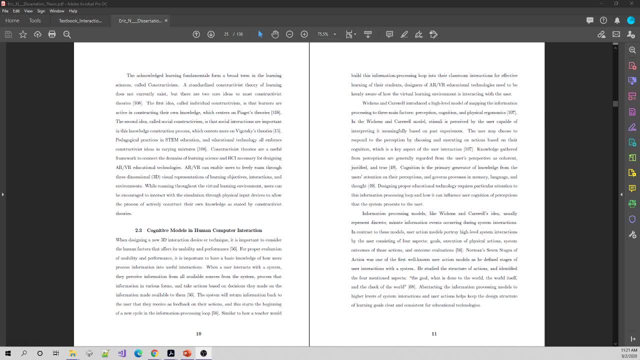 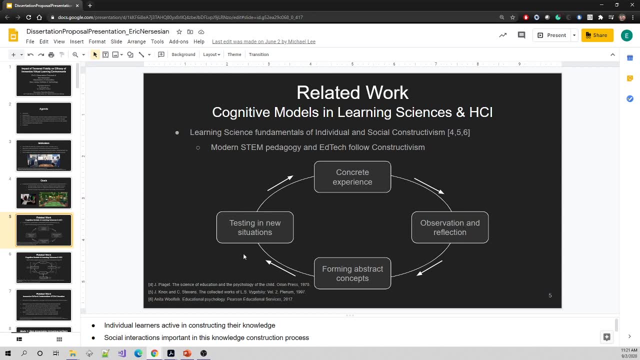 So if I open, let me just find that one window again. yeah, So you can think about this from the individual practicing. so trying new code, new interaction ideas, trying to think about these educational theories and then apply them in an area that you like Say: oh, I really loved eighth grade biology. I want to do a little sample lesson. 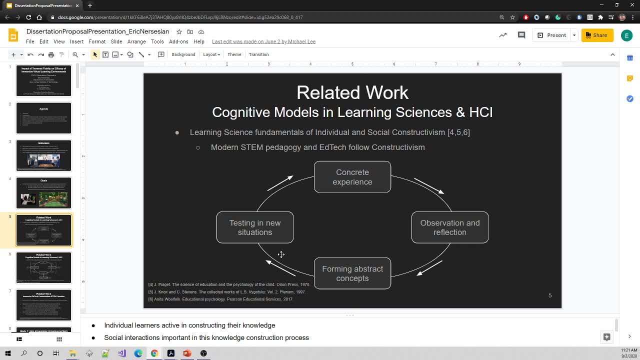 in there or whatever. Now, that's from a individual constructivism, the PIEGO, the PIEGET perspective. or you can think about students interacting with others and trying to form their own ideas and verbalize what they've just learned to somebody else, to their parents. 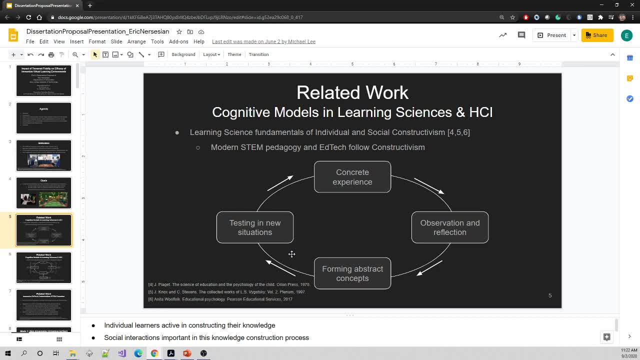 to their friends, to their colleagues in the classroom, to kind of ground themselves in the knowledge and they start to learn, and they start to learn, and they start to learn. And then they start to learn in a social way, in a cultural way, And that also is this section. 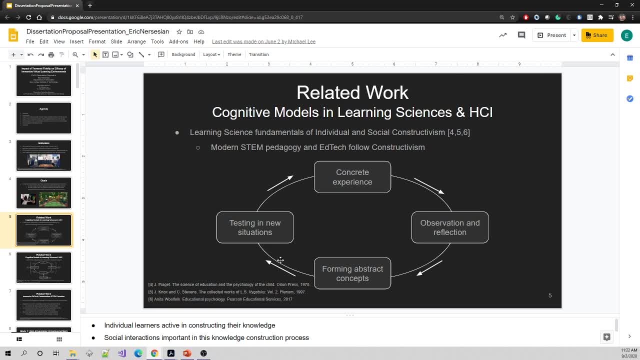 They're practicing the knowledge, but in a more cultural or social way. So there's many, even just looking at these two, an individual or social perspective on cognitive constructivism or just cognition, the process of learning. You can look at it from the 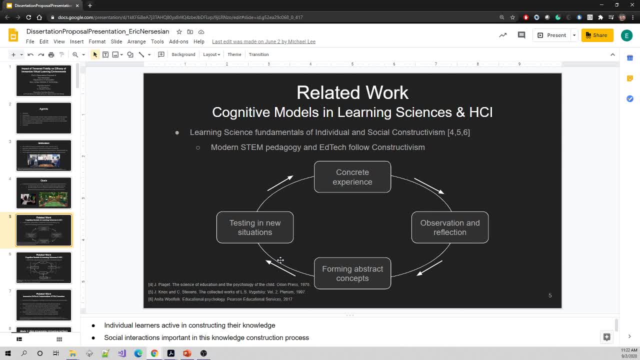 teachering side. You can look at it from the learner side, But it's a lot of different things And it's important to always kind of have two: I's the individual, I the social I, because you can't avoid our cultural. there's no person, there's no I. you know, it's we and the person. 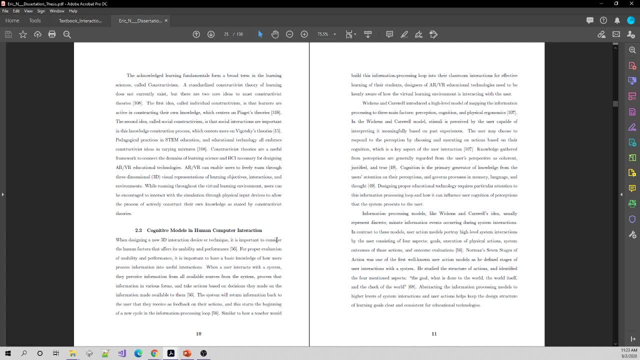 And that's just our reality. So let me move on. So another section in Related Works talks about cognitive models in human-computer interaction. So I kind of briefly show you that user system loop. But now I completely, I try to approach the ideas of education, learning from a psychological, a person, a human-oriented side. 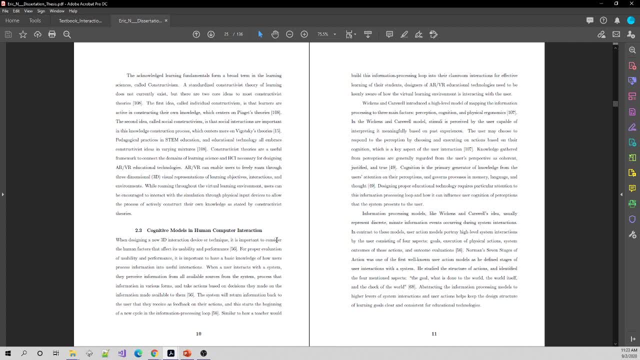 And this section actually tries to approach the software side, software and hardware, the computer side, the technology side, the educational technology side- from the psychological, from the human-oriented side as well. So if you are interested in HCI or UX, you'll hear these terms a lot. 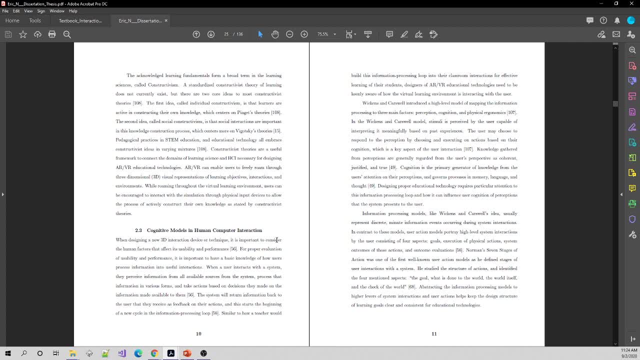 Human-centric, human-centered, human-oriented. In fact, the term human-computer interaction in the field focuses on the human side. when a person interacts with a piece of technology, with a computer, There's no point to any of this technology, any of these computers, without how they're aiding. 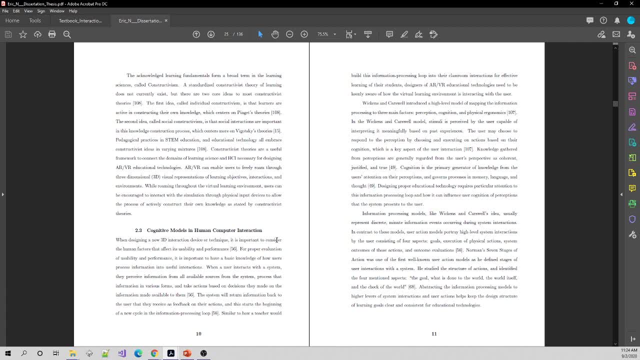 interfacing with the human. So it's a big part of it as well, And that's why we have these feedback loops as graphics, as ideas to talk about education and to talk about technology together- edtech- In this section I kind of covered this all with, I mean HCI side. 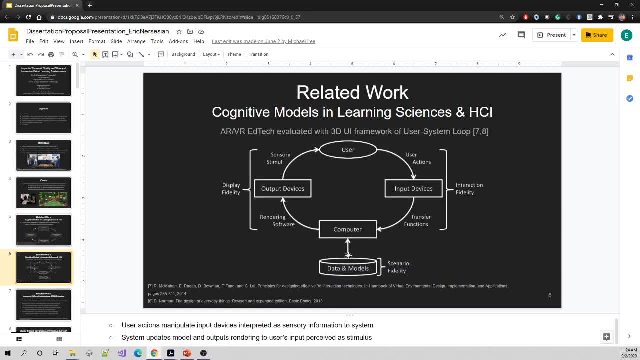 I'll probably talk more in a. Yeah, I'll probably cover this more formally in another section, But this being the first week, I kind of glazed over it. There's the user, the human, the psychological side. You produce actions on the hardware. 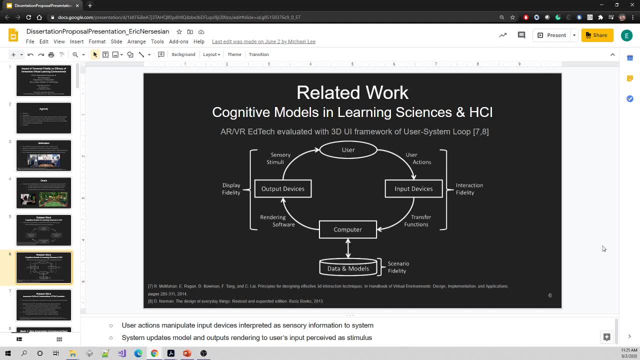 The hardware sends, transfers that information into something that's useful for the computer to manipulate the simulation, to update the visuals and audit audio, and have to through hardware output devices, back to the user And we cycle, cycle, cycle. I mean all this might be happening in a very small fraction of a second. 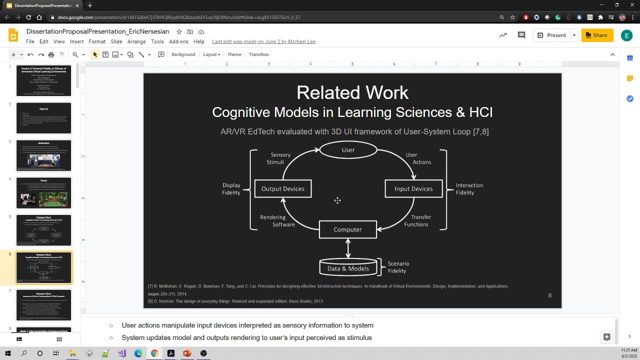 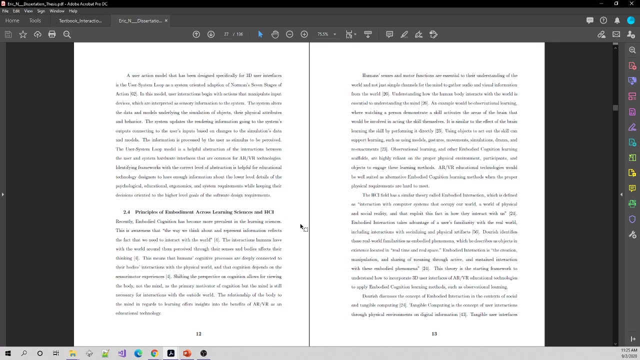 So the user sees this as a continuous seamless process. But the monitors and the speakers are all processing out very discreet movements that are so small and quick that over time the user feels like a seamless experience. So I just moved to the next page. 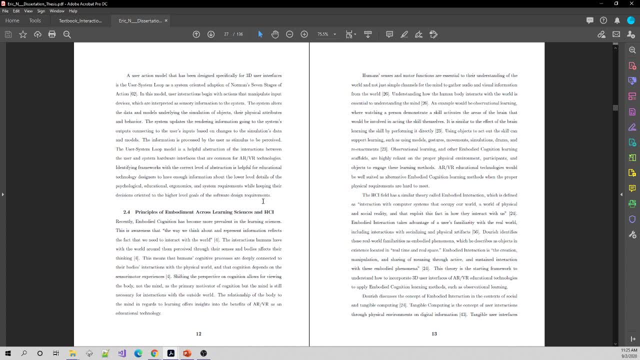 Principles of embodiment. Okay, so this actually might be interesting to talk of. I talked about this, about the stronger benefits of AR and VR, But let's talk about this for a little bit. So we talked about: you can't separate the mind or the individual person from the learning experience. 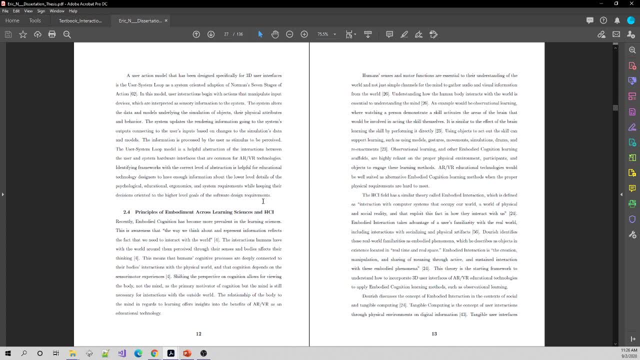 You can't separate their culture, their social surroundings from the learning experience. And now this says you can't separate the body. So embodiment, and there's a term in the learning science called embodied cognition And there's a similar term in HCI called embodied interaction. 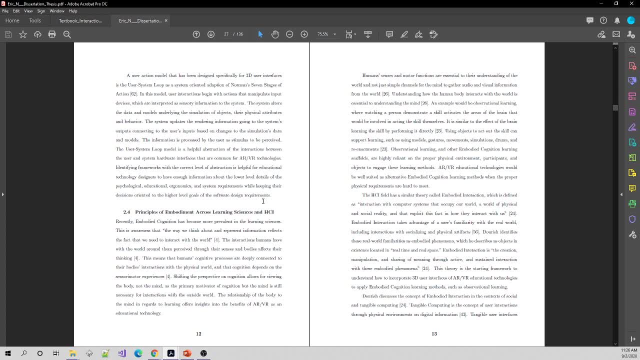 And so this idea of embodiment means that everything we're talking about- if you notice all my rants- talking about these physical processes dealing between the computer hardware, the person, these electromagnetic waves and the deciphering of what that means through all these cells. 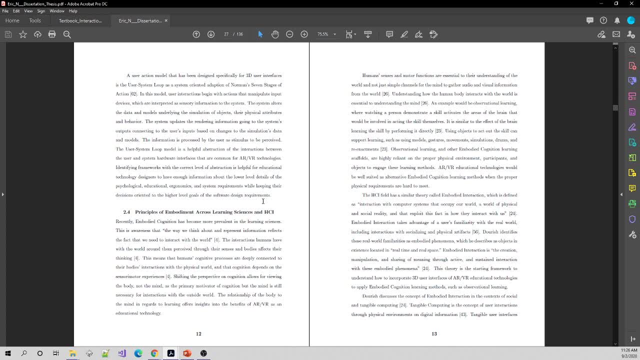 and the sensory organs of the human body through to the mind. we're talking about this idea of a physical reality. All of our learnings are really about this. what's going on around us? What is this world And what am I in it? 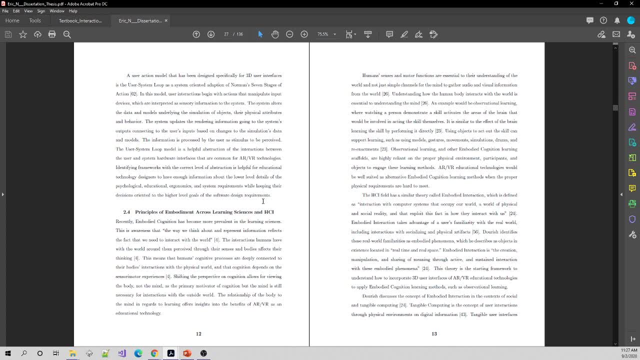 And what do I need to learn to function within this physical world, this natural world, this human world? And you can't really separate this idea of a body from the learning process And from the computer interaction process. Learning is in depth with the sensory information. 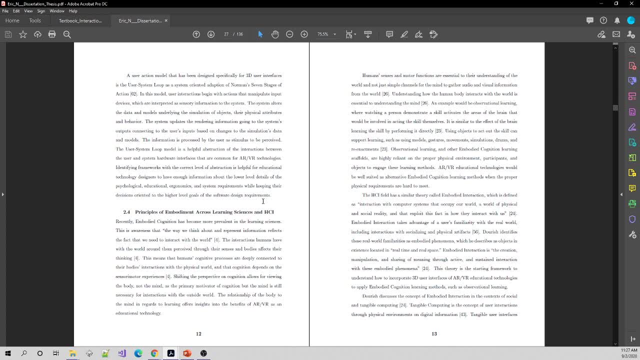 Again, the eyes, the ears, the nose with smell, the whole skin with feeling. And feeling might be broken down into like temperature and humidity And pressure, the feeling of gravity and what have you. So we have this idea of embodied cognition in learning sciences. 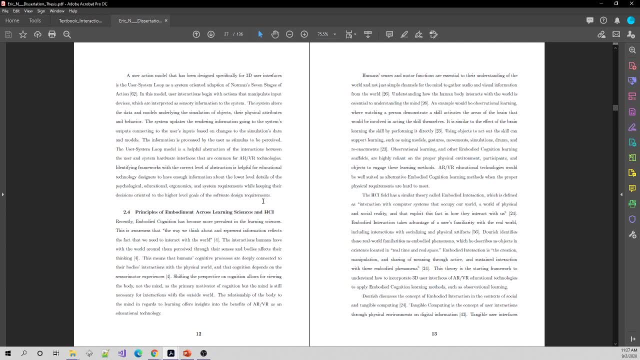 that you must think about the body and learners' physical surroundings and their physical body when approaching a learning topic, And even in topics as abstract as mathematics and computer science and physics, but even a science like biology. I mean, we're talking about cells in the body. 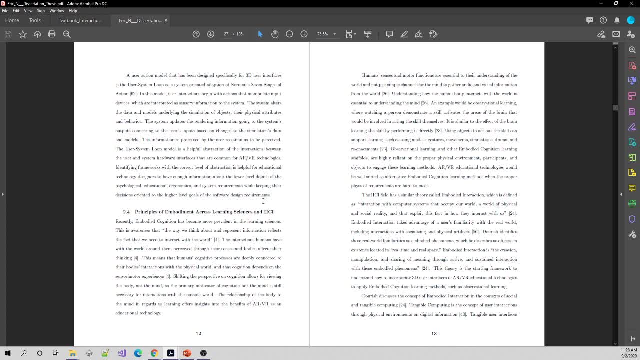 It's imbued in the topic. But think about moving to areas of applied sciences like engineering, mechanical engineering, chemical engineering, industrial engineering- and thinking about moving to trades like woodworking or auto repair or carpenter. These are learnings that are more hands-on that you must. 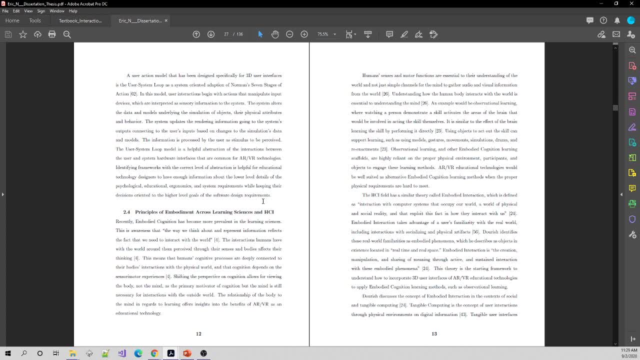 you can't just sit there and watch. You should never. you can't do that in any learning discipline. But there's no way you're going to learn to be a carpenter without understanding how to use your hands. Our musician, our artist. 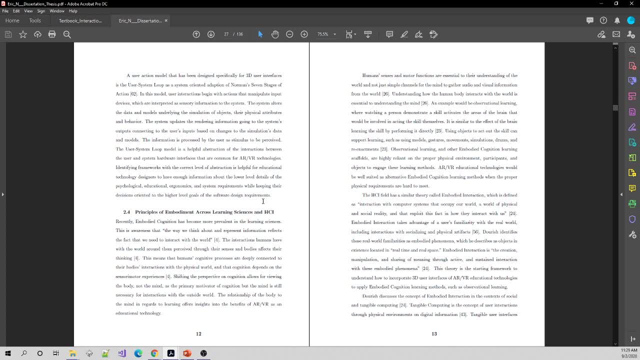 or anything any type of, I guess, if you look at learning, where you're trying to give them a career or something to do like gardening or sewing, which you might not think as a career, but it's an activity that you can't pull away from the hands or the body. 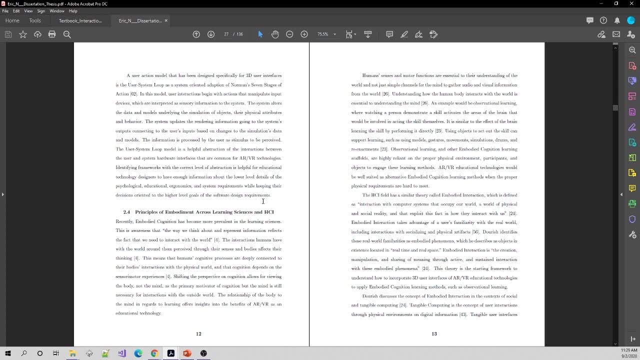 All of these learning topics are like even reading: you think there's nothing to it And you see it. You still have to understand how to move your eyes across the page. You still have to understand how to flip a page. You still have to understand how to hold your body. 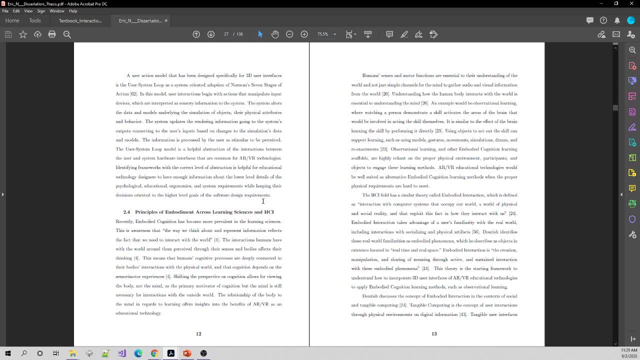 as you're reading, ergonomics, so that it's comfortable. All of this comes into the play as well. So we have this interesting connection between learning, science and HCI fields as well with this principles of embodiment. So I just talked a bit about embodied cognition. 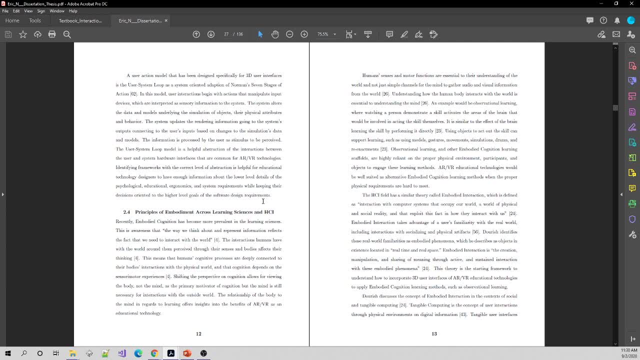 And you have to think about it as you're developing education or learning scenarios. but now across into the field of HCI, is this idea of embodied interaction, So interacting with computer systems that occupy our world? I'm over here right now And again we have this world of a physical and social reality. 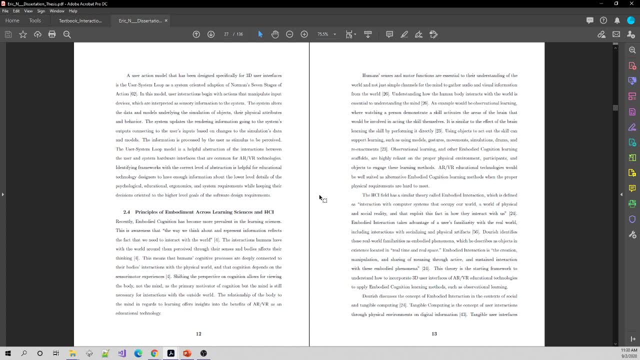 and we're always going to be interacting through it with the learning process and just life itself just happens to be in this type of reality. So all of our learning and education and technology use cases have to be there as well, And so embodied interaction is kind of a broad, loose term. 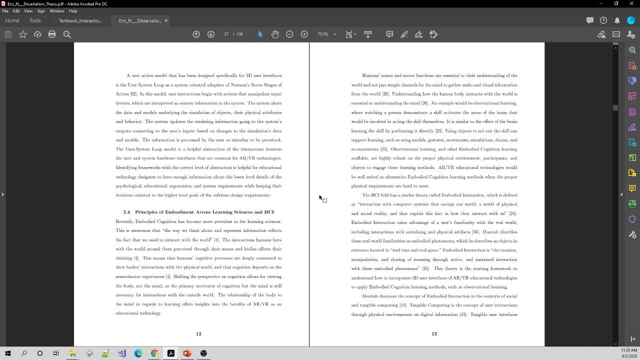 It can mean a few things. It can mean like: oh you have this computer system set out where physical objects in the world actually interface with the computer system. So if an elevator is run by some type of embedded computer system actually pushing the buttons on the elevator, 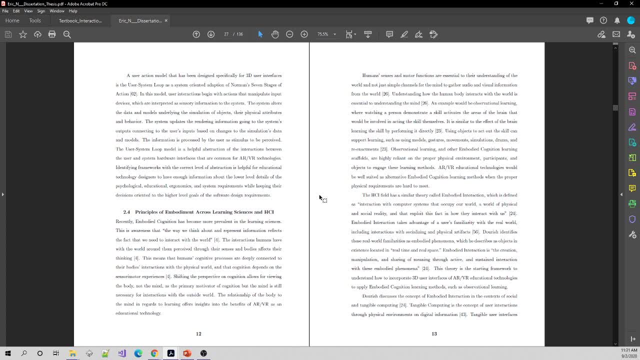 is embodied interaction, Because you're thinking this is a physical object, I'm pushing it, I'm going to go to floor two. But when you push that button it's sending some type of signal, some type of computer system that is running the elevator system. 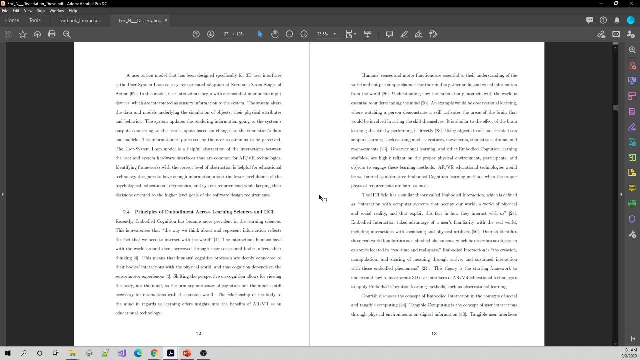 So you're actually interfacing with a physical object, that is actually interfacing with a computer system which these days it's getting harder and harder to step away from it. So even like the low front of your refrigerator might have a digital display. 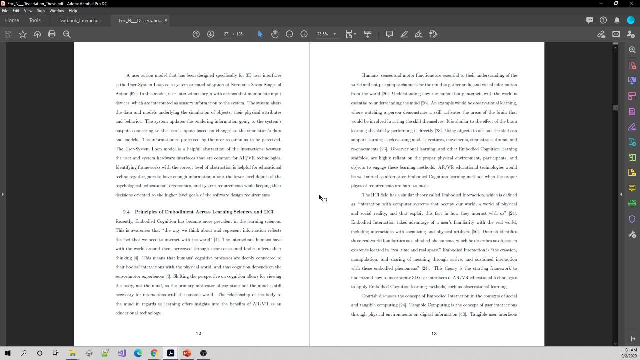 and you can change ice cubes to water and you push your glass on that lever and it releases either water or ice chips. Most of these systems might be purely mechanical, not have an electrical or computer system come onto it many, many years ago. 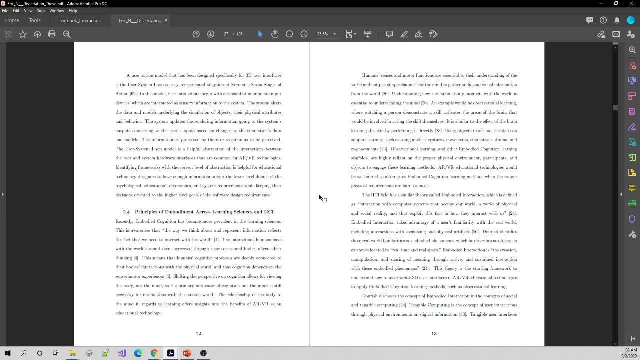 Now, a lot of these things have small computer systems, these embedded computing systems. That's why Internet of Technology, IoT, is such a hot field, And this is you're interacting with a physical object which is interacting with a computer system. 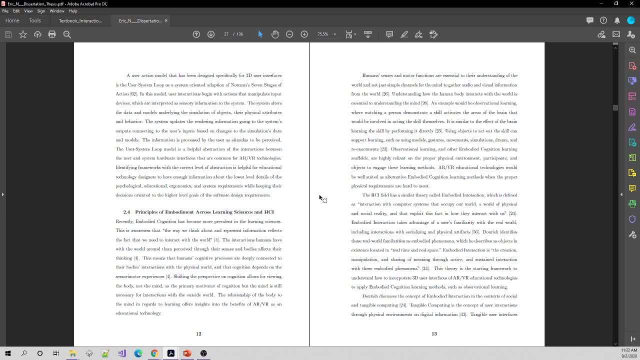 But there's another part of embodied interaction. Now think about you're manipulating physical objects. They could be virtual representations of physical objects. So I'm just going to bring over one other slideshow quickly. This is the BIOS. This is the BIOS. 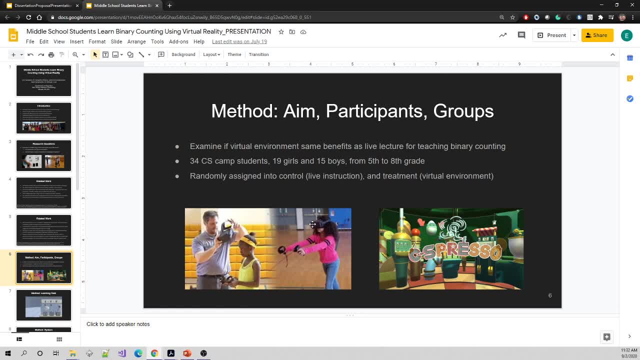 This is binary math, But if you think about the fact that the student is in virtual reality with this hand controller, now you don't even need controllers, just the basic hands. but they're kind of grasping at nothing or they're grasping onto this piece of technology. 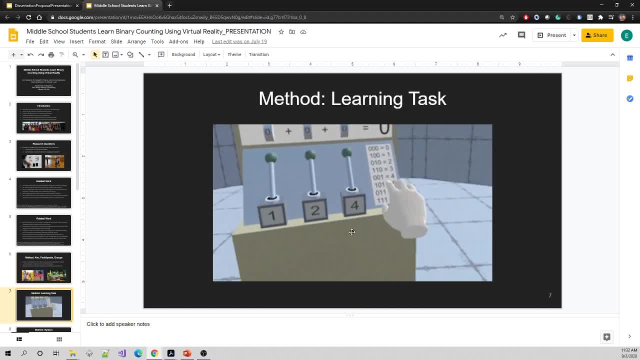 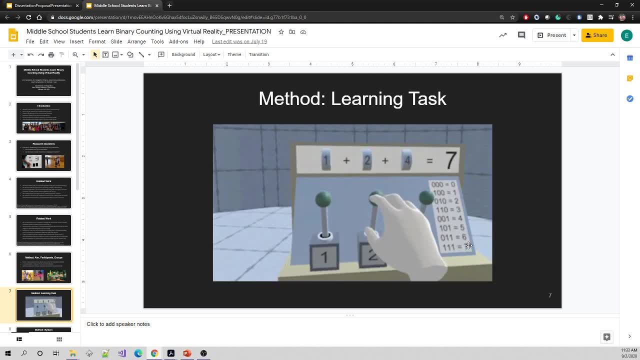 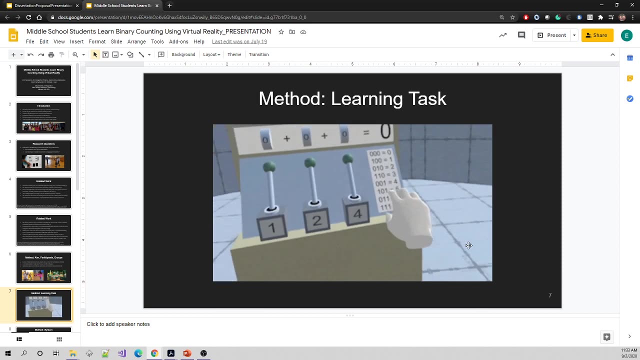 that doesn't have anything to do with what their brain is processing as reality. So if you think of this term as embodied interaction, but if you put them in a VR headset and they get immersed, meaning they think that the virtual reality is their real reality. 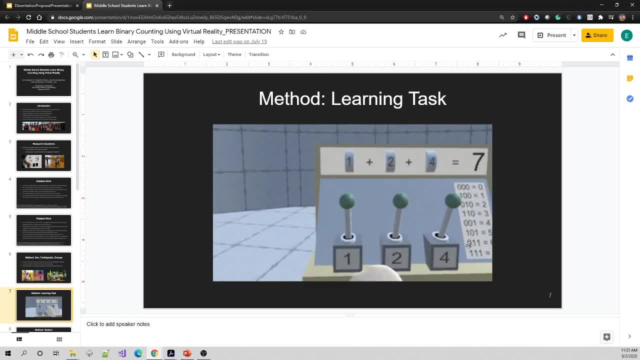 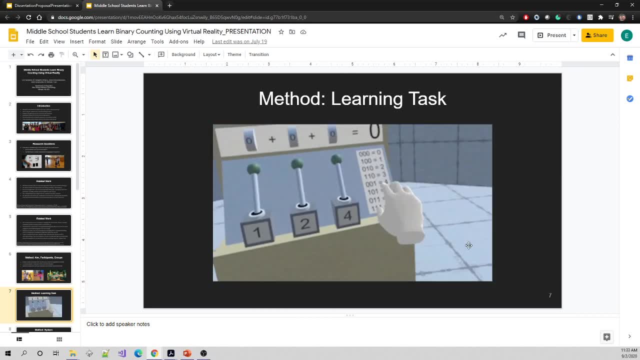 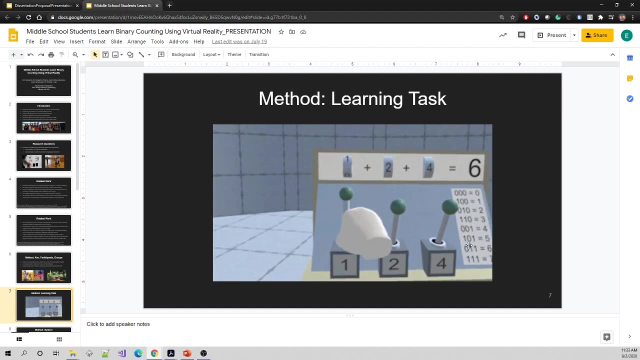 then whatever they're interacting with, which looks like physical objects in virtual reality, is actually an embodied interaction. They're using their virtual hand to pull a virtual lever. I just don't feel like building this whole system in real life. I don't want to make this room. 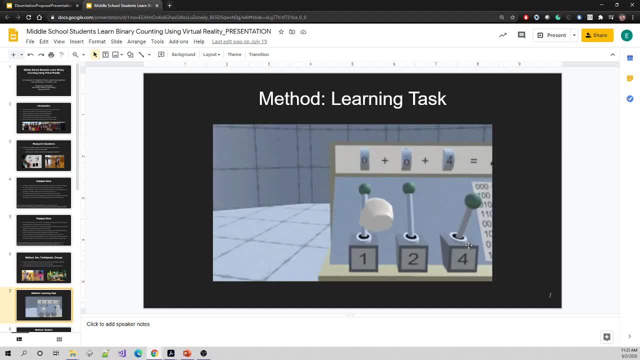 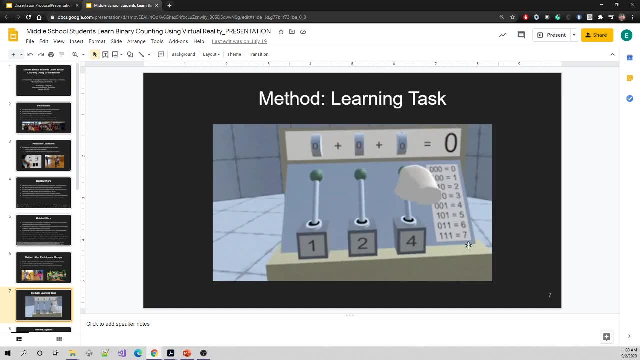 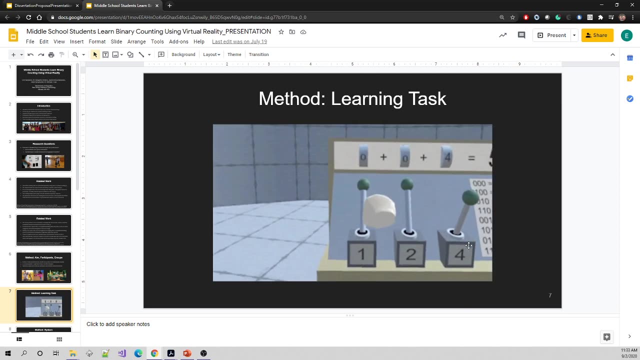 full of all these computer systems and levers to teach them about binary counting. It's much cheaper and quicker for me to build the virtual representation, a simulation of it, but the user thinks they're in the simulation, so we can also use this idea of embodied interaction. 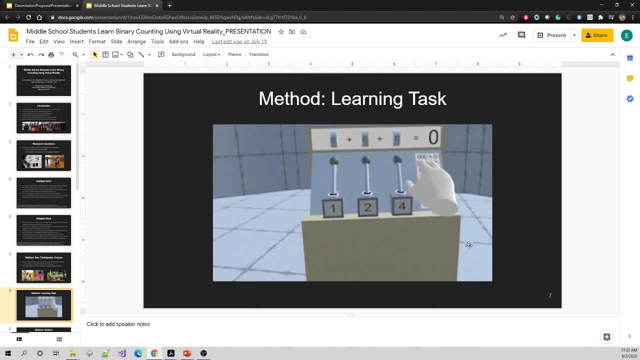 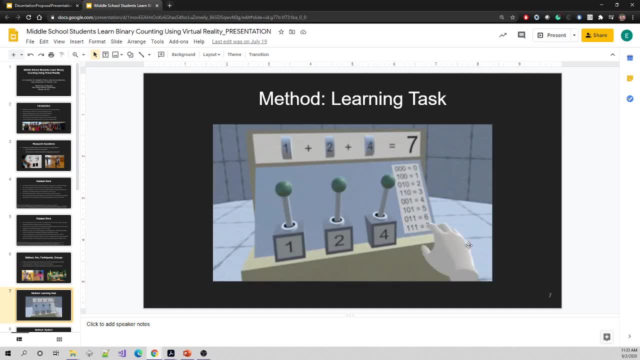 I'm using my body to learn something abstract. So I think this plays really strongly into the fields where it's mostly abstract- computer science or what have you- because learning abstract topics can be very hard for people and we're very comfortable interfacing. 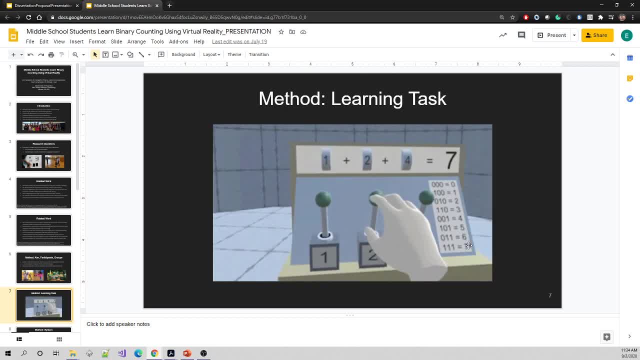 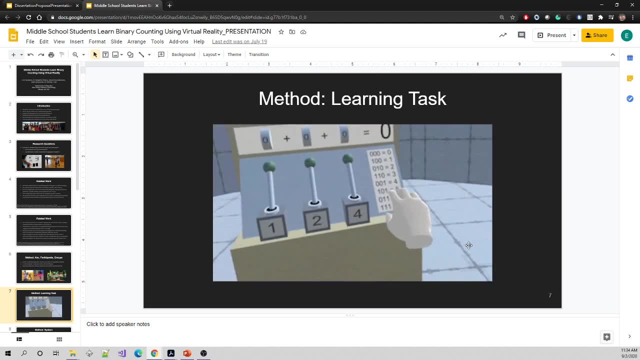 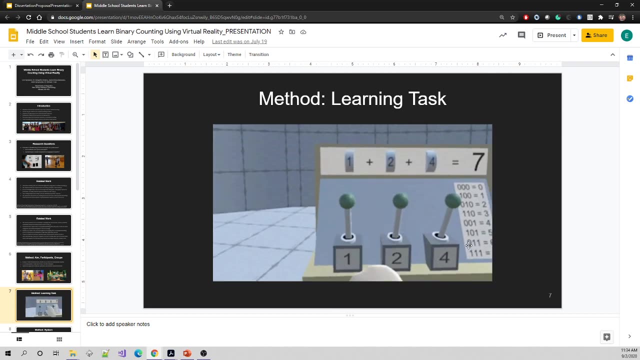 interacting and thinking about the physical reality, our physical world. So any way you can represent an abstract topic in a physical way and give them an embodied way to interact with it, I think it grounds the knowledge. Now, this is all. there's not a lot of research done on virtual reality. 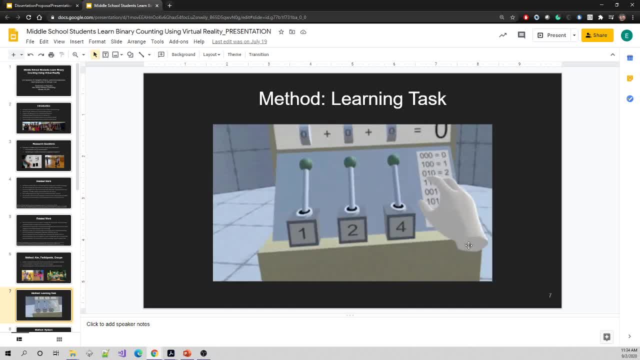 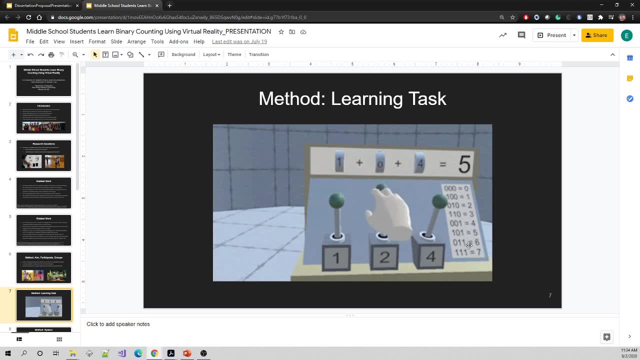 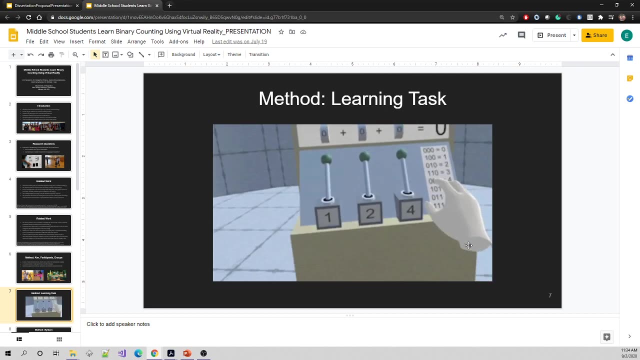 and education itself. always, anything about psychology is going to have multiple opinions because it's just such a vast and unknown field, And so I'm going to state that these are my opinions, but I can say that we used to have great results with teaching something abstract. 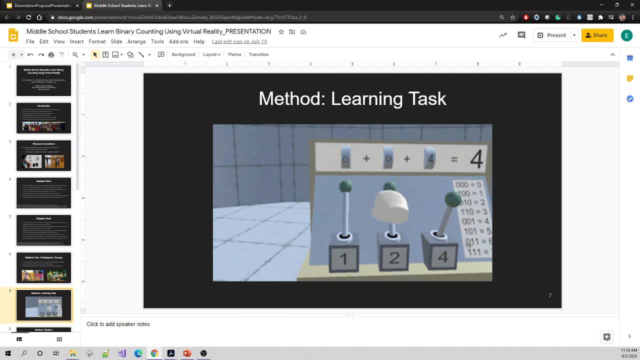 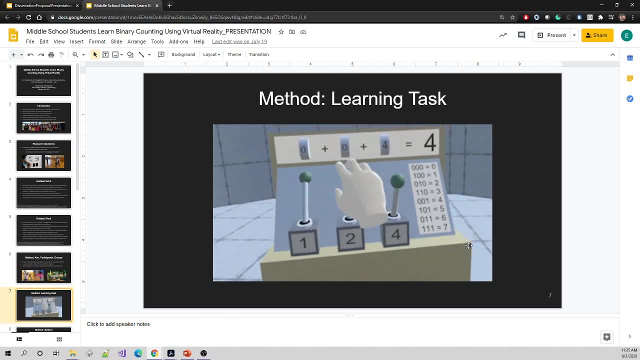 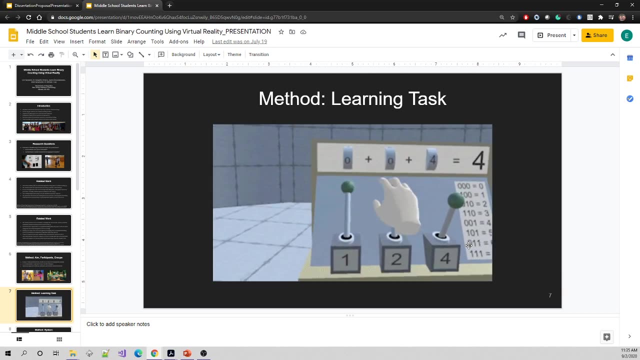 the fact of binary math, how to count in a binary format and not a decimal format, how to look at a string of zeros and ones and how to convert that in your head to decimal, or an idea of a certain amount of numbers, giving younger students almost a play world. 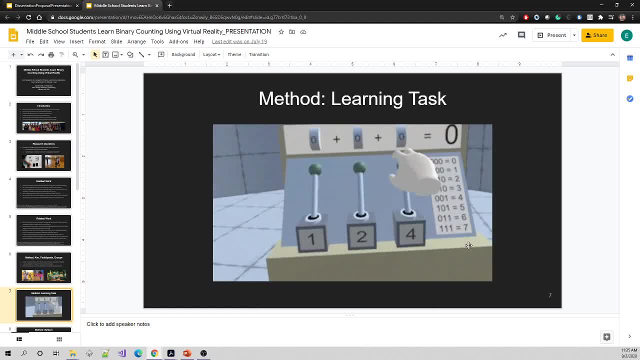 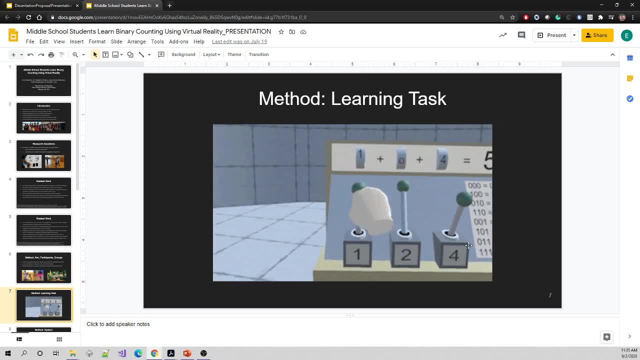 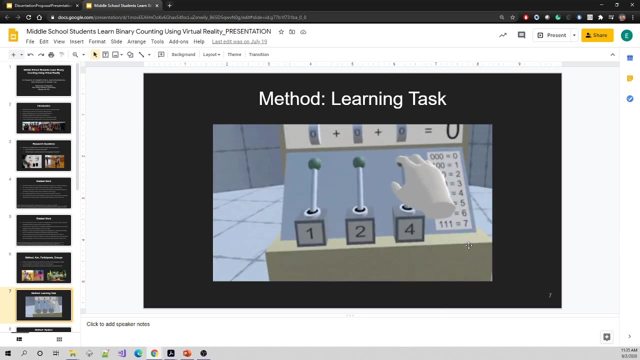 a illusionary physical reality where they can interface physically: pull levers, push dials, push buttons, turn dials- what have you? gives them a much stronger feedback loop, If you think about the learning loop, basically giving embodied interactions or interfacing with physical reality. 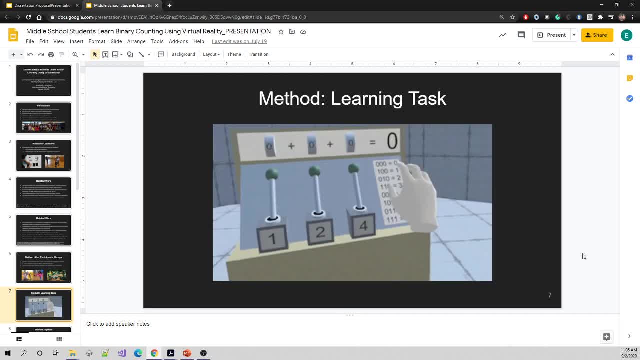 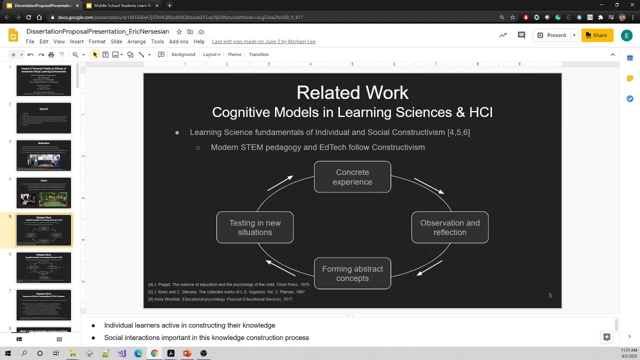 which, psychologically, we're very accustomed to because that's our world. I think it tightens this loop super fast And I think the more you loop on a concept of learning and practicing- learning and practicing- you're refining your, your neural network, your neurons. 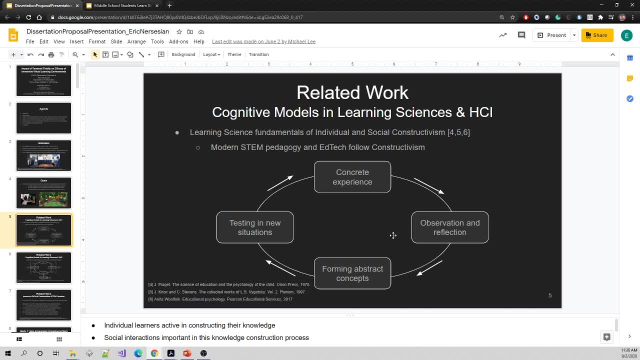 their connections. that gives you these cognitions, these thoughts, helps you refine them much faster, And so this idea of embodied interaction, which is on the HCI field, I think lends itself well to embodied cognition, which is on the learning science field. 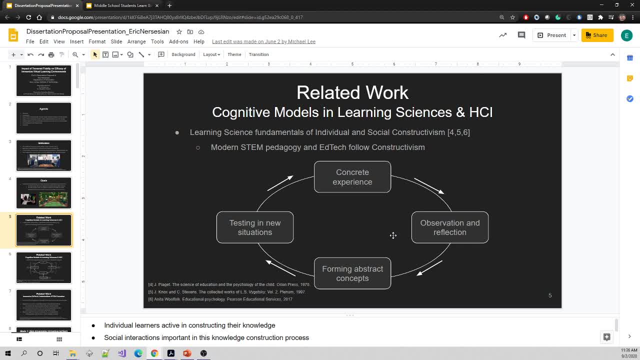 but the whole idea that you can't separate the mind from the learner, you can't separate their cultural pinnings, underlyings, background, socialization needs and wants from the learner. And now you can't separate the idea of the body. 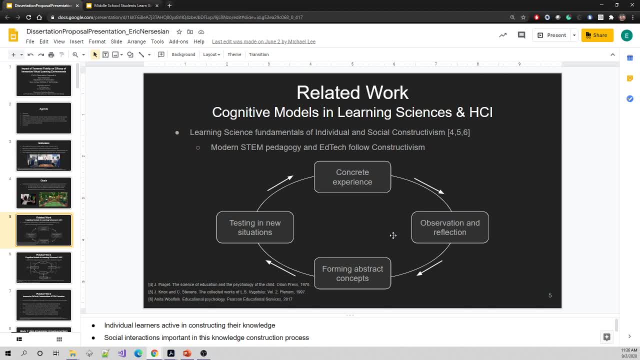 You can't separate their body from the learning experience, and you shouldn't. And so you're kind of sitting in your chair. You're listening to me. It's very passive mentally. This is very passive body-wise. That's why it's not lecturing. 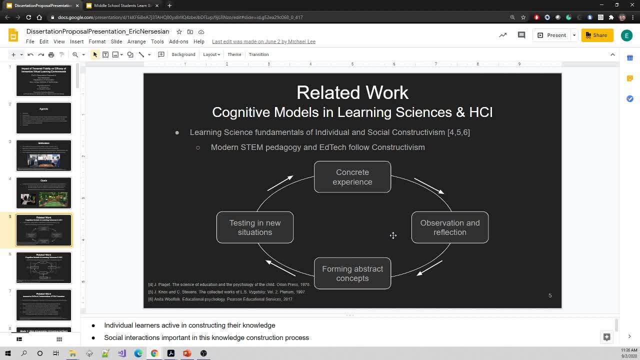 It's not always the best way to get information across. It's just right now. you know, in a physical classroom I can't kind of interact with you. This is the most I can kind of interact with you. But I'm just saying that embodied interactions. 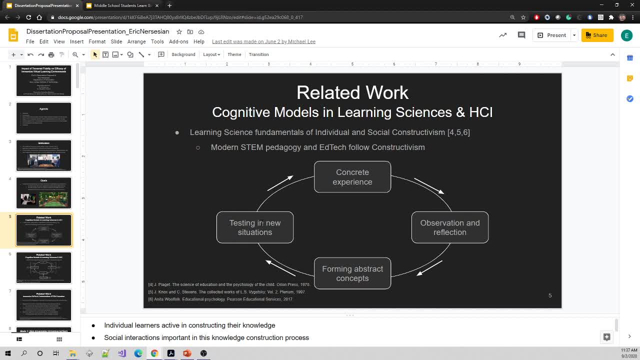 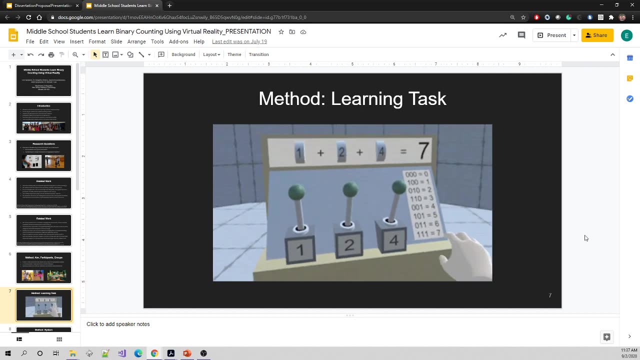 I think, tighten this loop because you get to practice much quicker on abstract ideas like STEM, science, technology, engineering and mathematics And anytime you can do a embodied interaction, and that's the benefit. that my argument, basically this is my argument in my dissertation. 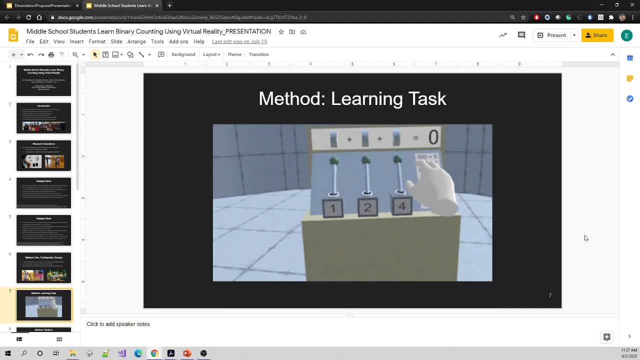 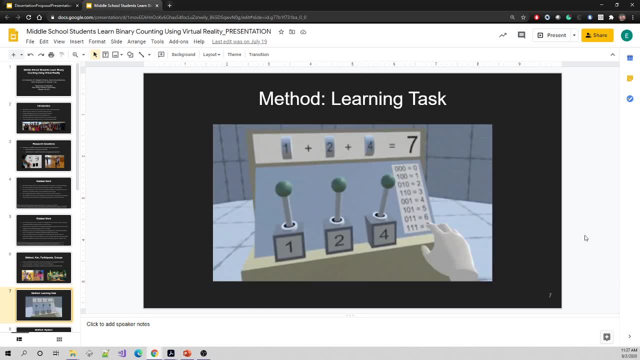 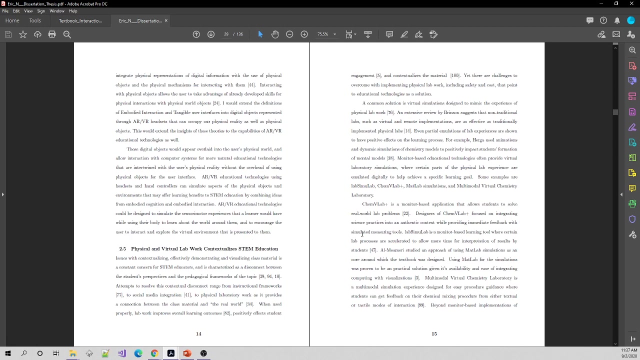 is that you can just get a better learning or better training experience by helping ground down abstract topics into physical activities to help speed up that feedback loop of learning. And that kind of relates to why the next section, like lab work, helps contextualize STEM education. 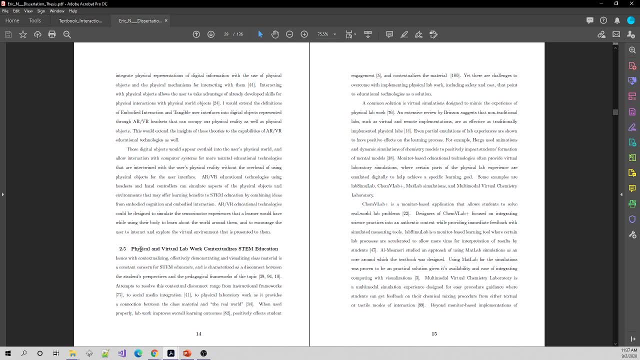 So physical lab work. so think of like using test tubes and beakers and doing like using the Bunsen burner in chemistry class to interacting with plants and animals and biology, and using the microscope on cells, on slides that may have cells or something else. 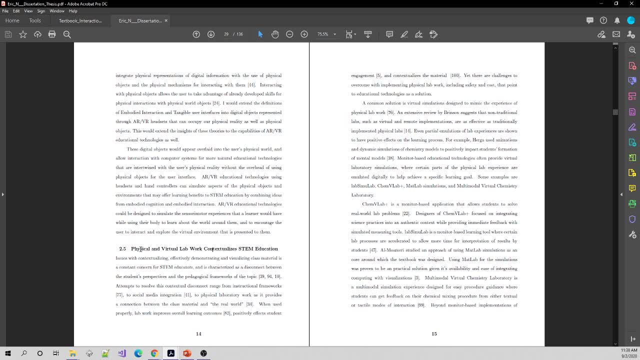 bacteria in it, to doing physical experience like throwing egg, the parachute with the egg off the roof or some other type of physical experiment for physics, to look at gravity and to even doing project work in computer science classes, And that's why lab work helps contextualize STEM education. 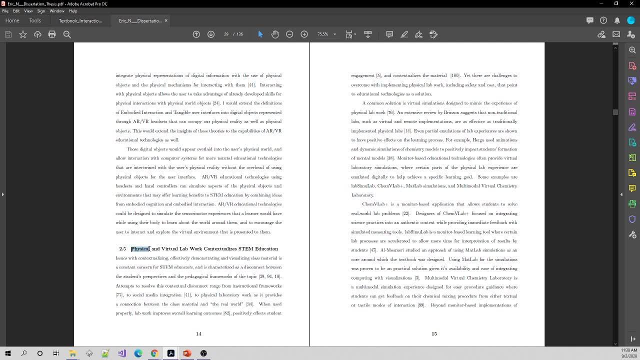 And the argument is that we traditionally done it physically but now we have so much advances in technology that educational technology can help replace all this lab work or supplement. it usually allow this educational technologies to supplement, So in this case we have a pandemic.